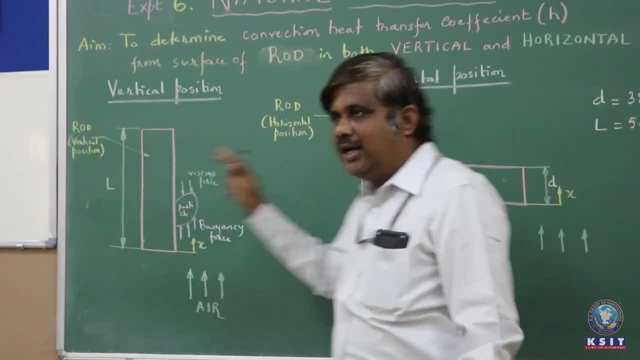 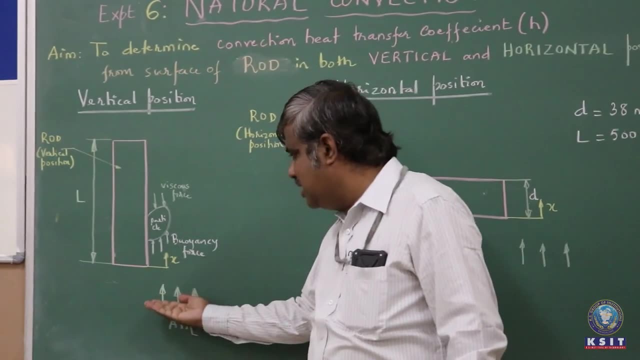 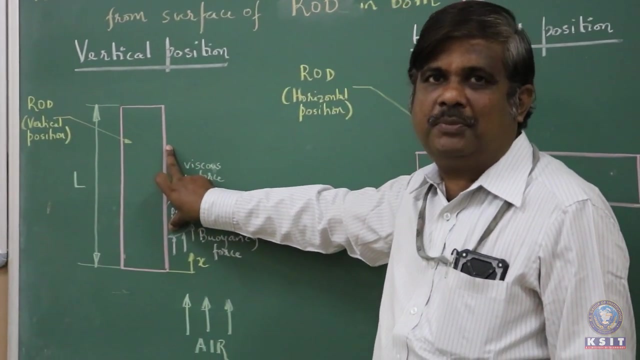 kept. We know the diameter and length of the rod as 38 mm and 500 mm respectively. and this is the hot surface and air is moving over this. The characteristic length is the length of the rod. I repeat: characteristic length is the length of the rod through which the entire fluid particle 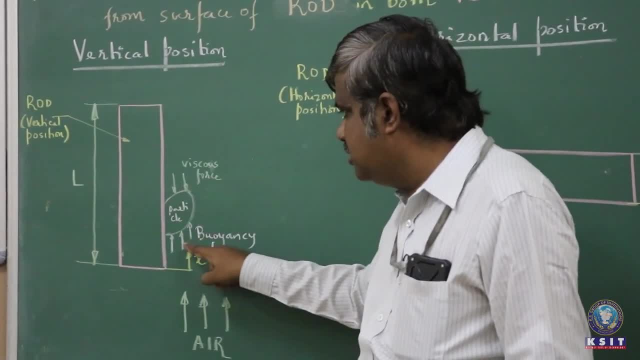 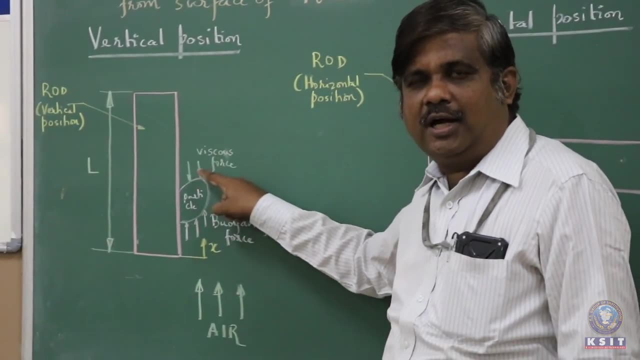 is been touching the surface. So the fluid particle will be exerted from underneath the buoyancy force and it has to overcome the viscous force and buoyancy force. if it is greater than viscous force, then it is a turbulent, and if it is less. 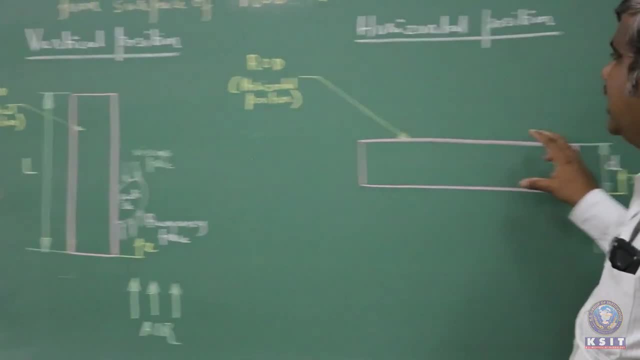 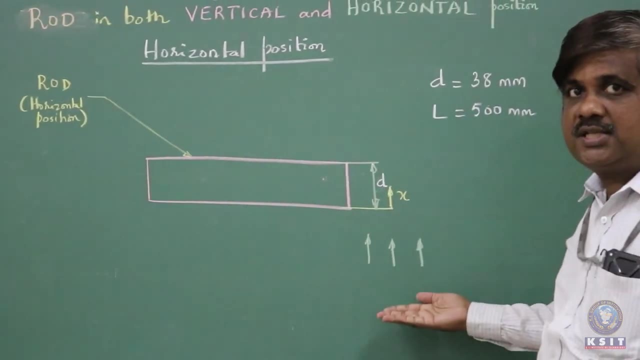 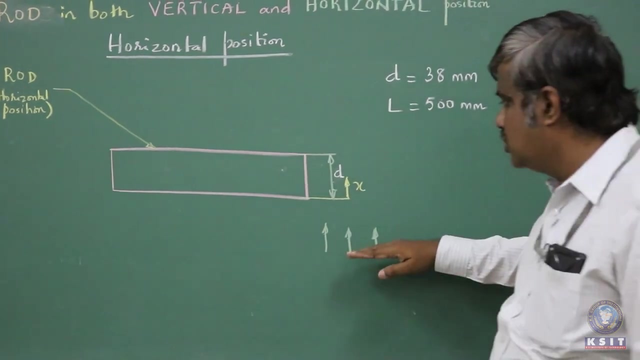 then it is a laminar flow. So the same rod can be kept in horizontal position. and can we can conduct the experiment. The rod kept in horizontal position, air movement is same, always from upward to sorry, downward to the upwards. So the air movement is always same. The 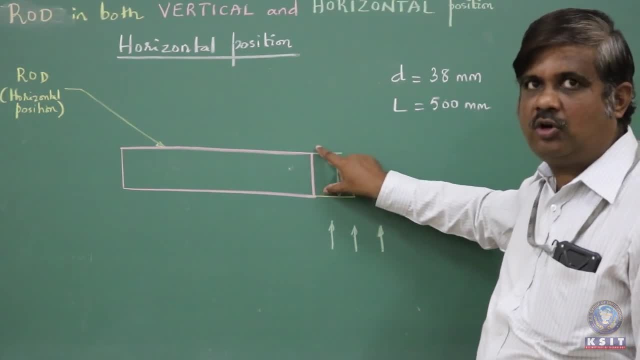 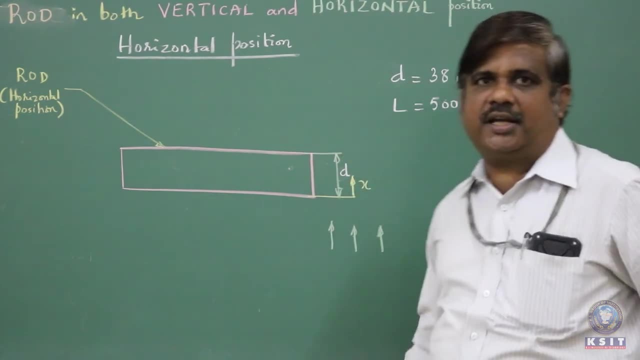 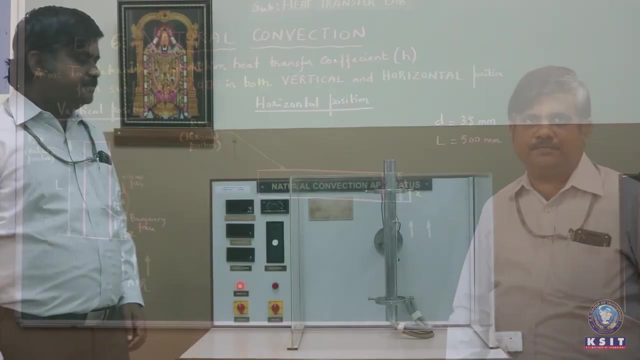 x direction is always upwards When the rod is kept in horizontal position. we have to take the diameter as the characteristic length. This arrangement will conduct the experiment. Now we will go to the equipment and see what are the readings we can definitely take. This is the equipment to conduct the natural 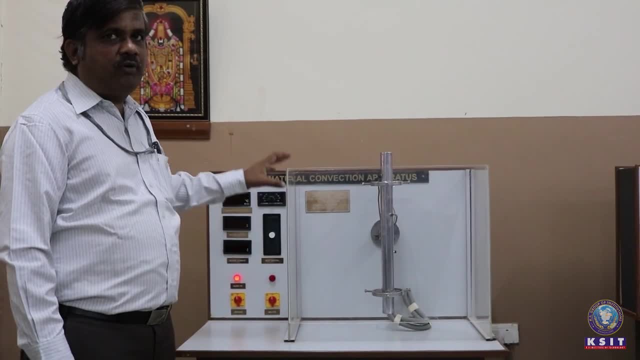 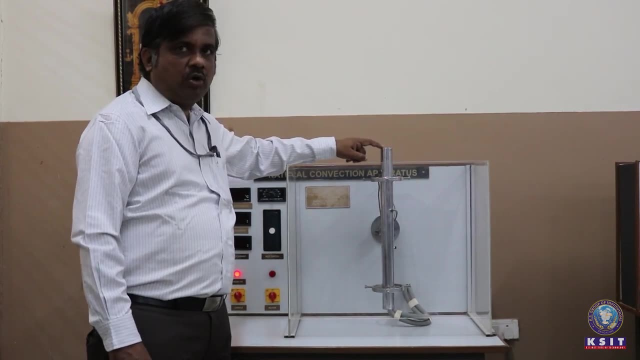 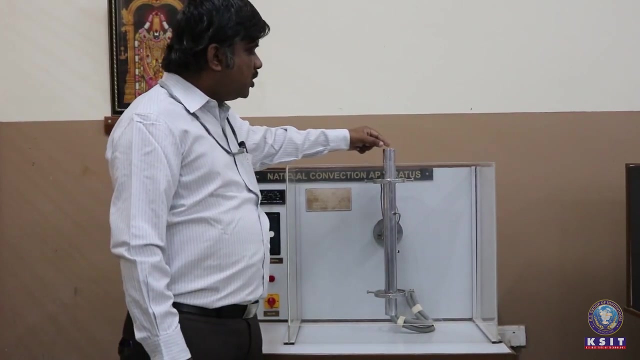 convection heat transfer and what we have to find from this is the heat transfer coefficient of this rod. The air is been passing through this hot rod and we have to find out the convection heat transfer coefficient by natural convection. So the diameter of the rod is: this is the diameter. 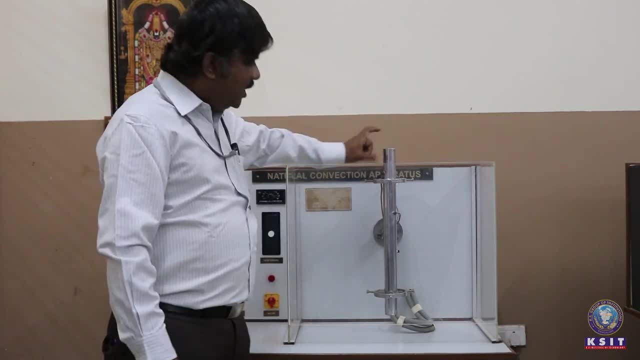 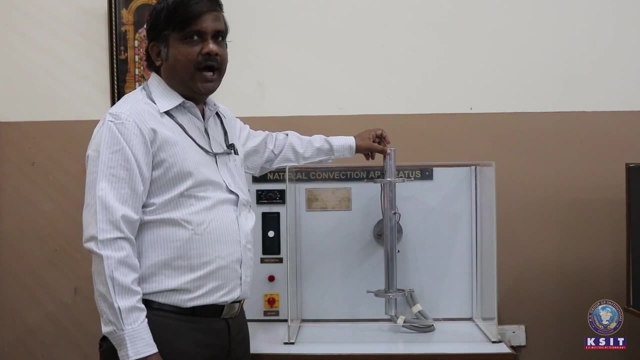 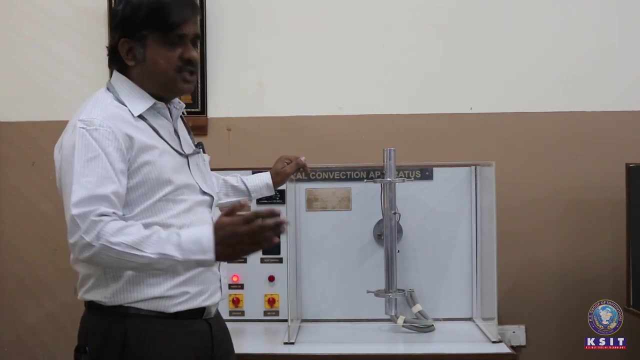 of the rod that is 38 mm. the length of the rod is 500 mm right and this is the hot surface. There is a heater which will heat the rod right and, since it is natural convection, we cannot have a blower or a fan to make the air to flow right. The air is flowing naturally, the air enters here. 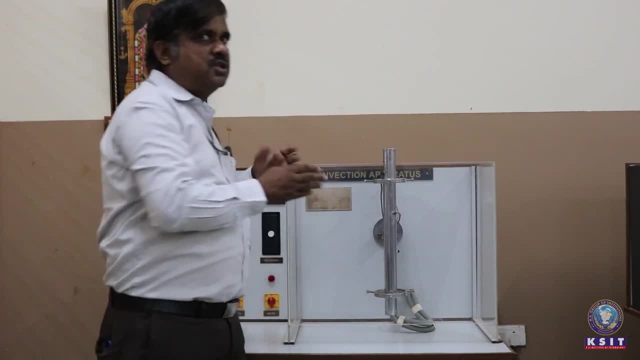 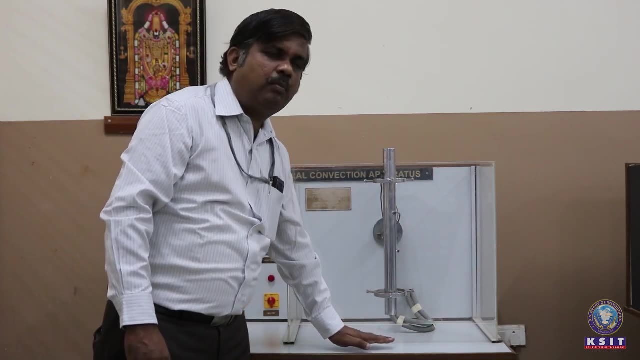 it moves upwards right. When it moves upwards, it touches the surface of the rod and takes heat right. So the air movement will always be from bottom to top. So this block what we can definitely remove this. this has been kept to. 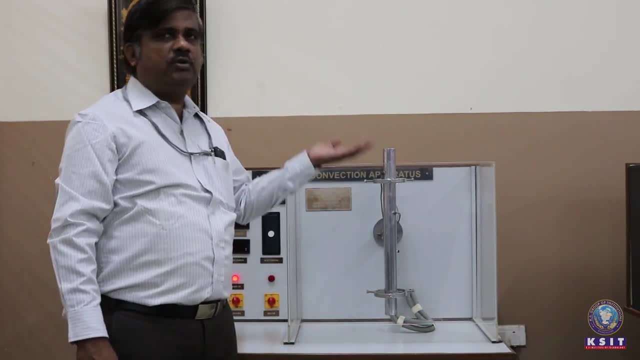 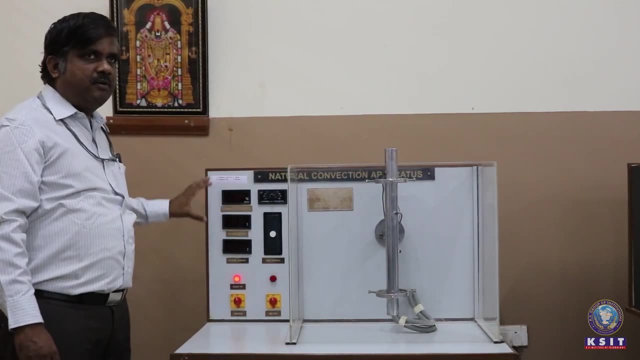 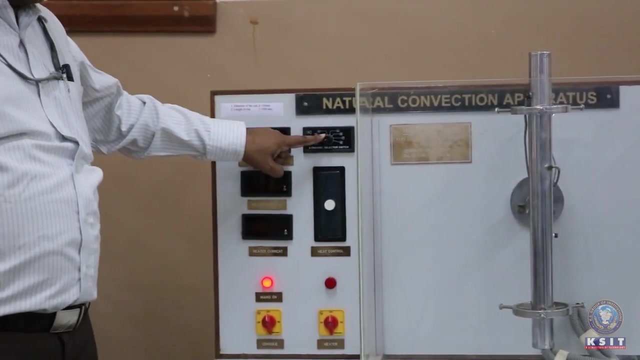 make sure that air is entering here and moving upwards and it is moving steady flow. It should always be in steady flow. So the accessories to take the readings are this: There is a temperature indicator, followed by the temperature changing switch. There is a voltage and the current. 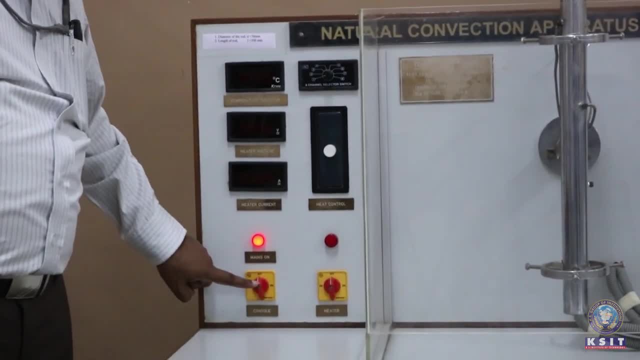 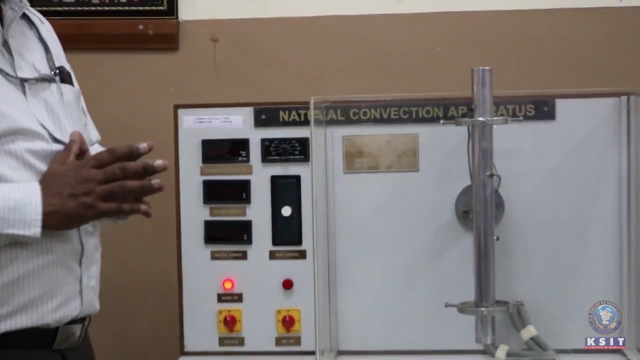 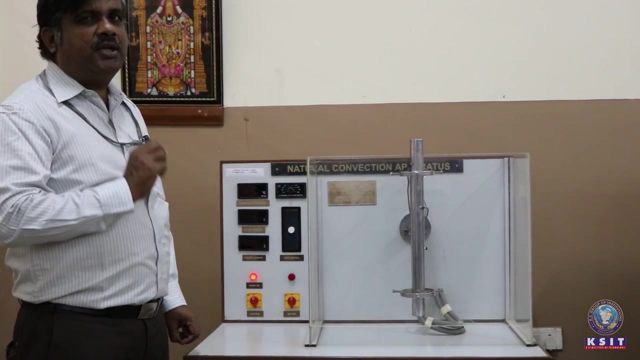 readings right, Then the console main switch. this is the main switch and this is the heater switch right. So first we will conduct the experiment to take the readings of keeping the rod in vertical position. I repeat the readings: what we are noting is by keeping the rod in. 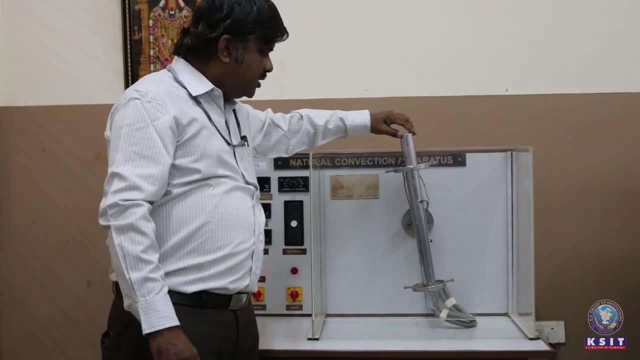 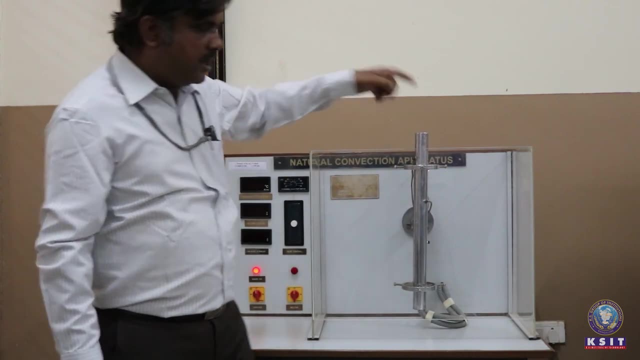 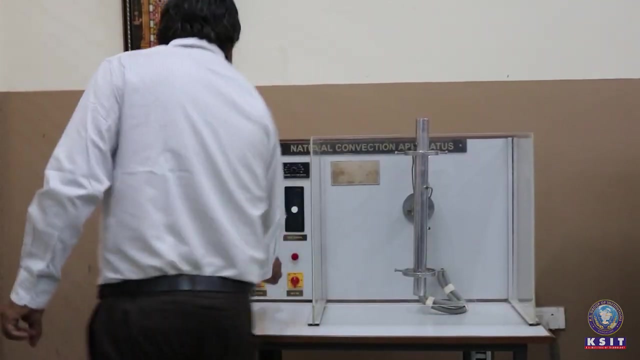 vertical position right. What is the step number one? We can rotate this, rotate this rod, keep it in vertical position right. Keep it exactly. vertical position. Switch on the main, the main switch here, Hopefully everyone can see this- The main switch right, Then the console switch right. 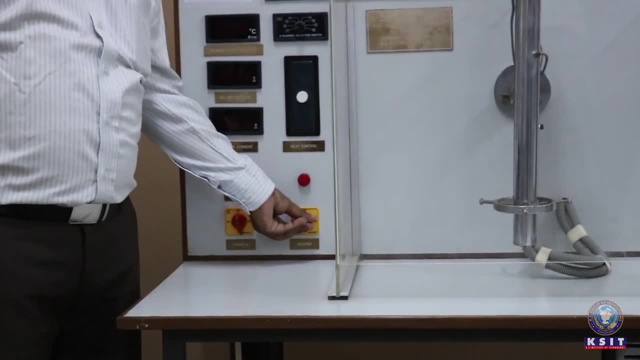 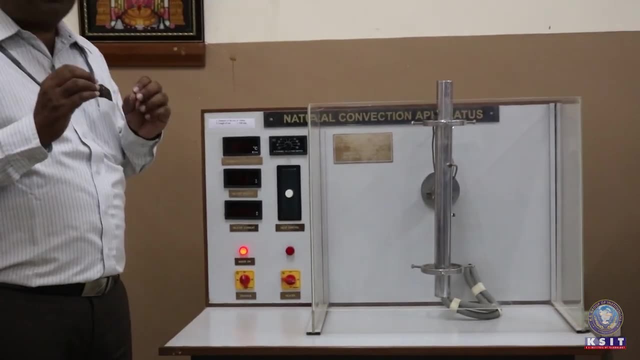 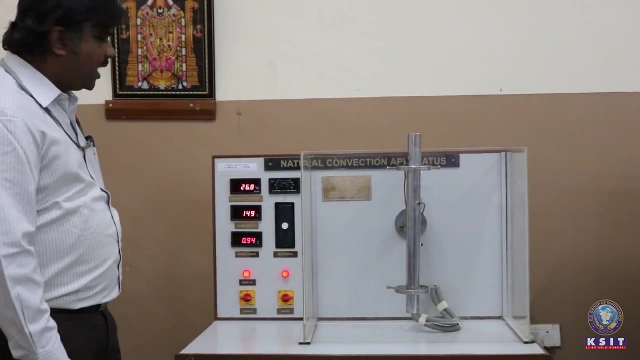 Then we have to switch on the heater right. Once we switch on the heater, there is transfer of heat takes place slowly, right After reaching steady state. after 10 minutes you can take the readings. 10 minutes has been done and now you can take the readings right. So what are the readings? 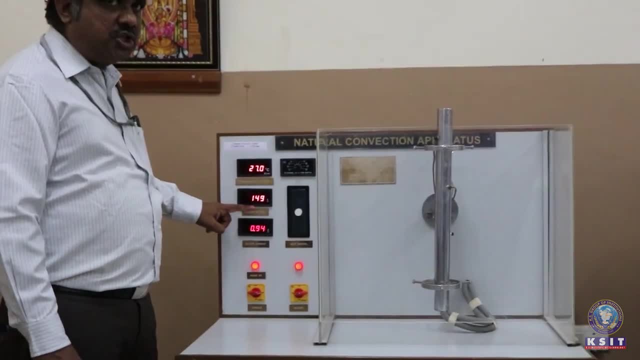 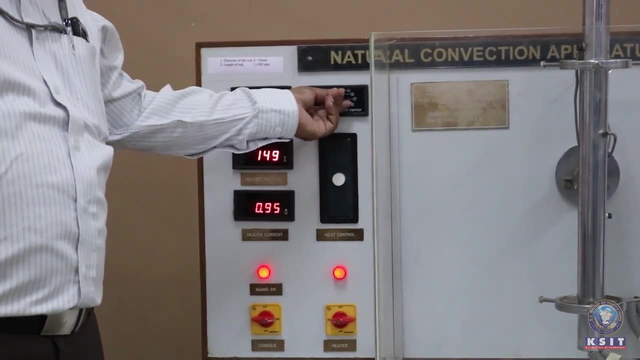 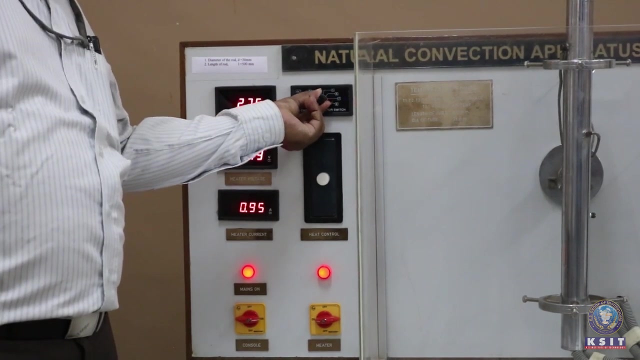 in the tabular We can check and take the values voltage, current right And T1, T2, T3, T4 are the four temperatures on the surface of the rod right. Turn this knob: T1, T2, T3, T4. This gives the four. 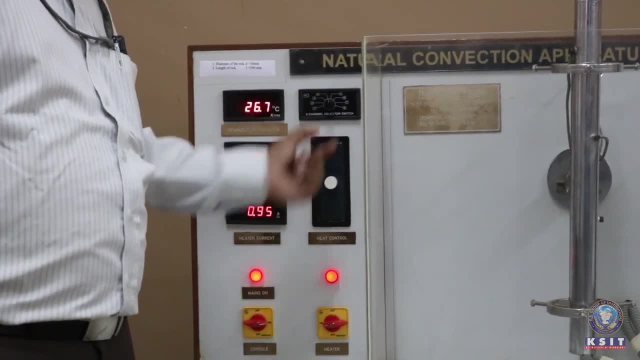 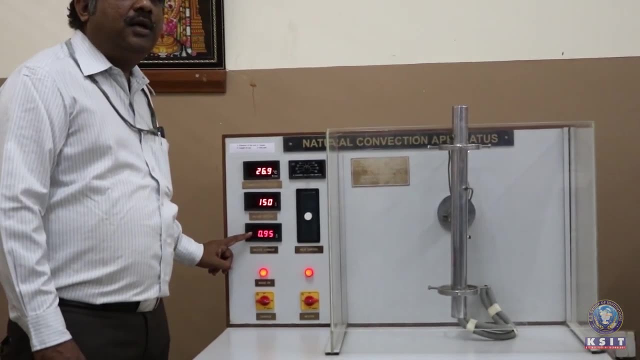 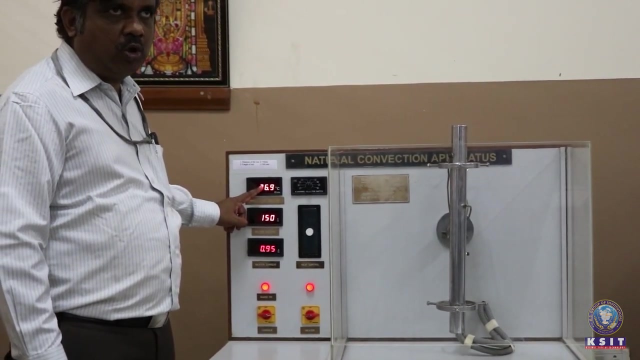 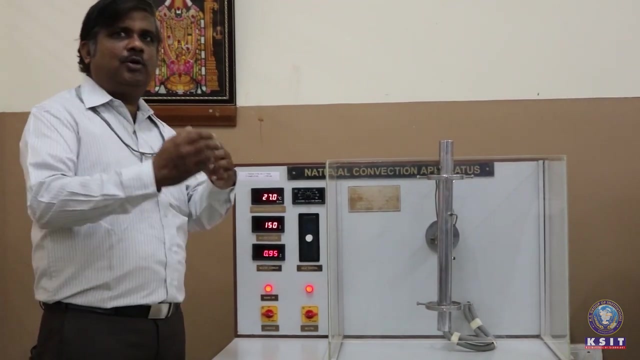 temperature values. Finally, the T5 gives the air temperature Only. this much is the reading Repeat: right The voltage current, Then five temperatures right: Four temperature exclusively for the surface of the rod and one temperature for the fluid. A right. So after taking the readings we cannot directly go. 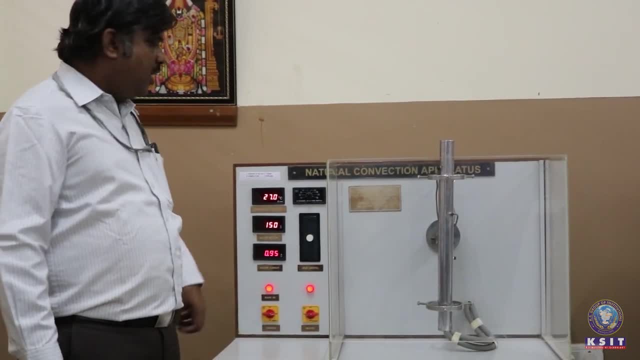 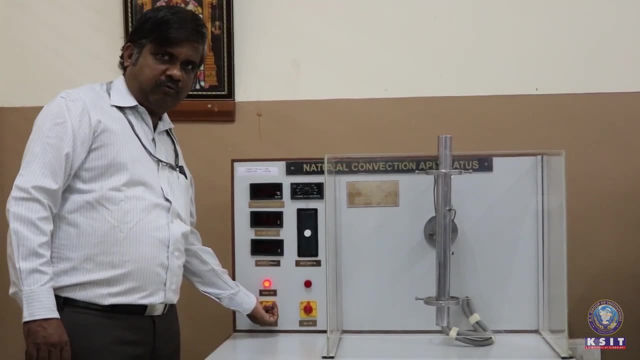 on to the calculations. We have to switch off this right. So by switching off, you make sure that the heater is off. the heater switch I am putting off now, right, And the main switch is being off, right. So then you can go back to the main and you can see. 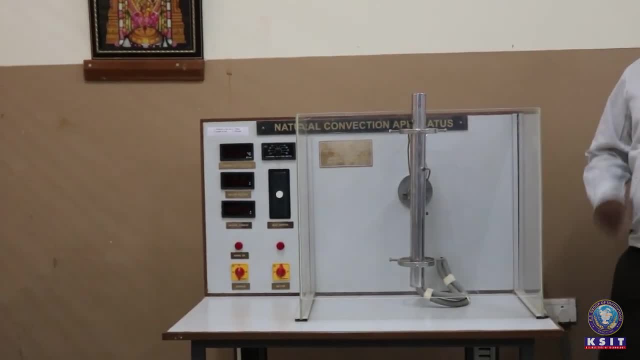 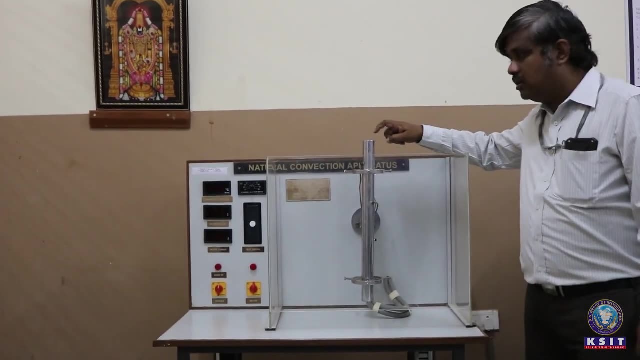 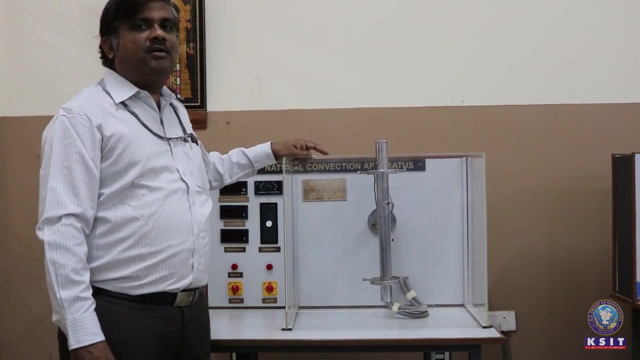 you can keep this power supplys off right. So this much we have to do: to take the readings for natural convection. keeping the rod in the vertical position. The now the experiment. what we are doing is the rod kept in horizontal position and 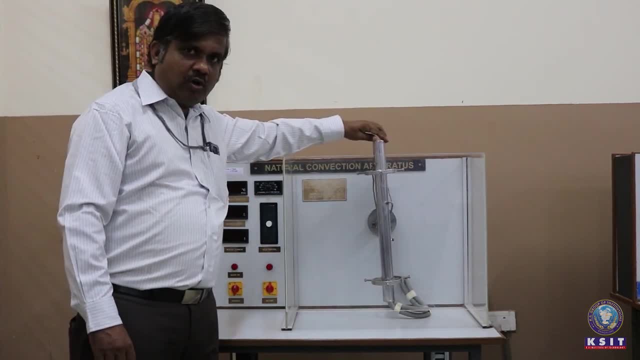 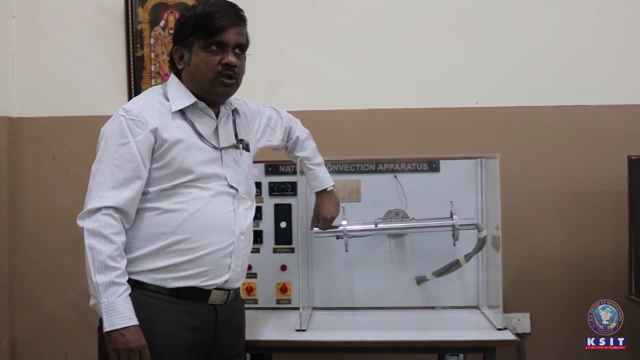 we work to conduct the experiment. Definitely we have to turn this rod to the horizontal position to take readings right Now I am turning the rod right And kept in horizontal in horizontal position. after keeping this in horizontal position, we have to switch on the main. 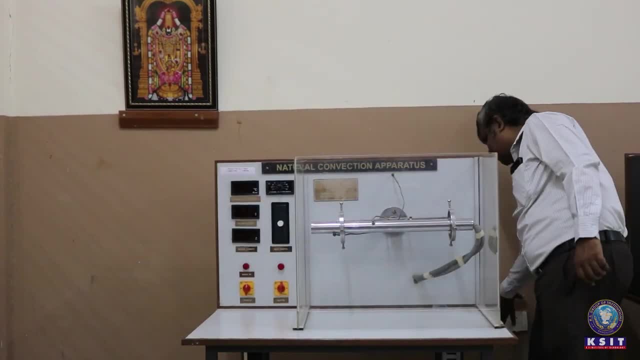 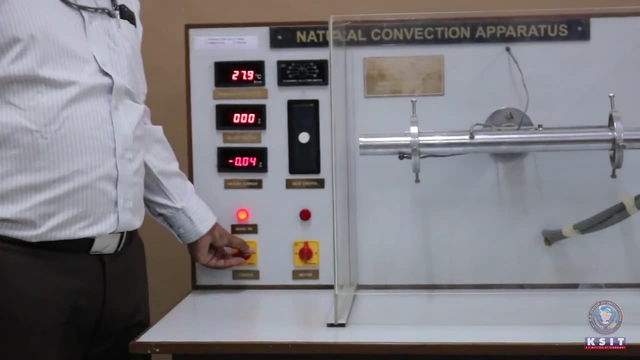 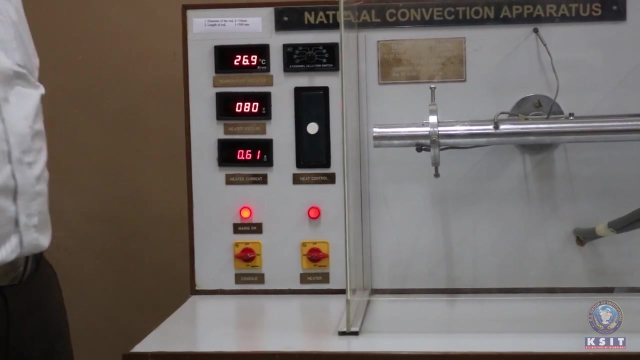 right, so i am switching on the main power supply now. right, i have switched on the main power supply now, the console switch being on right. further, the heater is being kept on right. so after switching on the heater, we have to wait for steady state again. right, that is, we have to wait for 10 minutes. 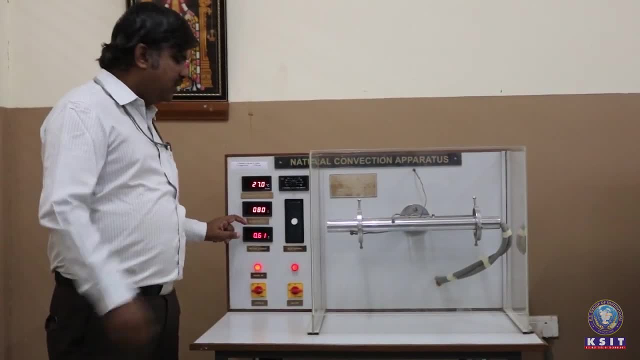 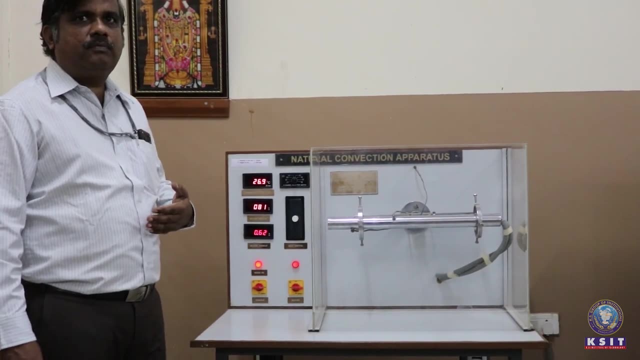 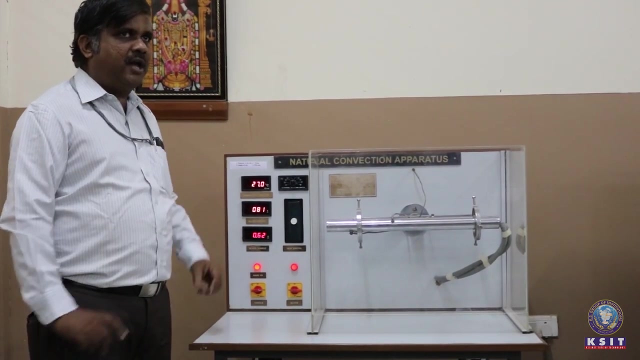 right after 10 minutes. we have to take this, the. we have to take this temperature and voltage readings right now. 10 minutes is done. right now we will take up the voltage and the current reading. right you can see the manual tabular column that has been available right: the voltage and current. 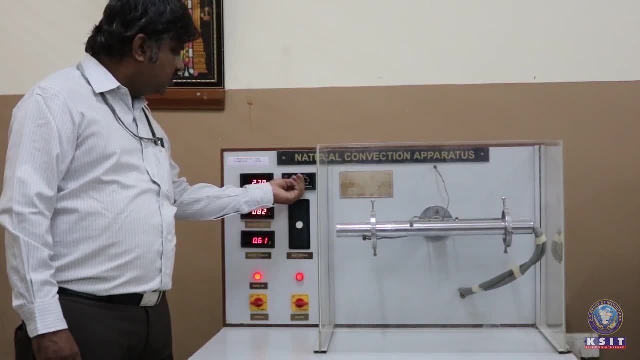 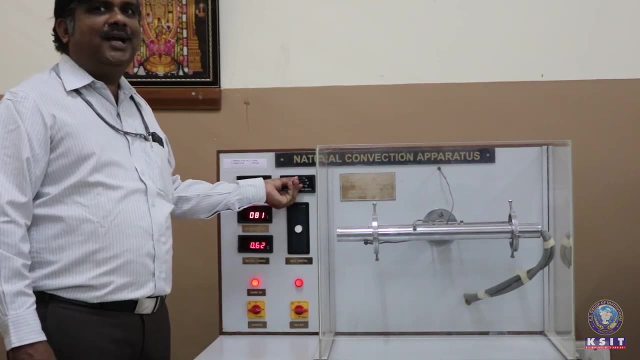 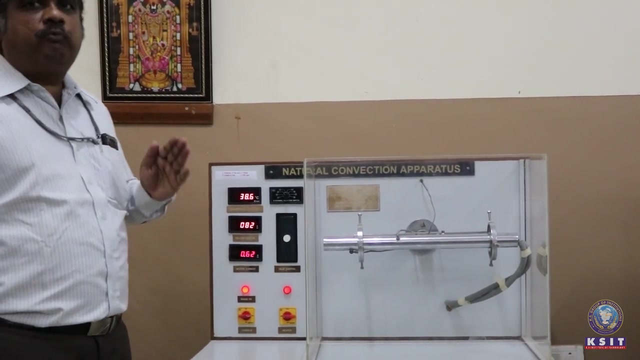 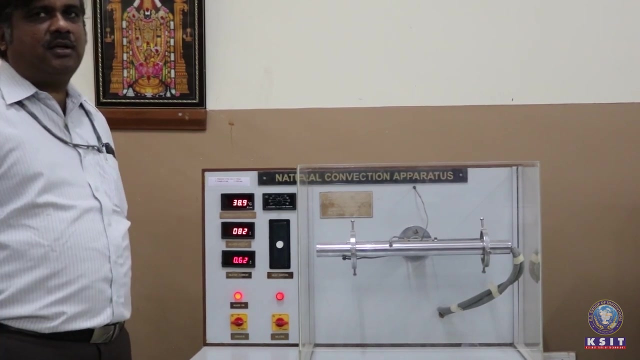 the first reading. right next, four temperatures, four temperature sensors on the surface, that is t1, T2, T3 we can get by turning this knob, and T5, the temperature of the air. So this much is the readings to be taken for horizontal position of the rod. So before leaving and doing the 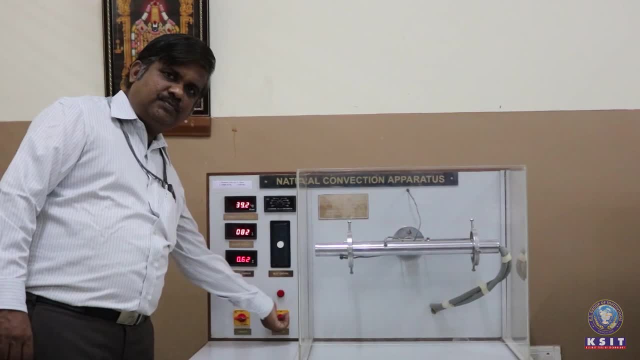 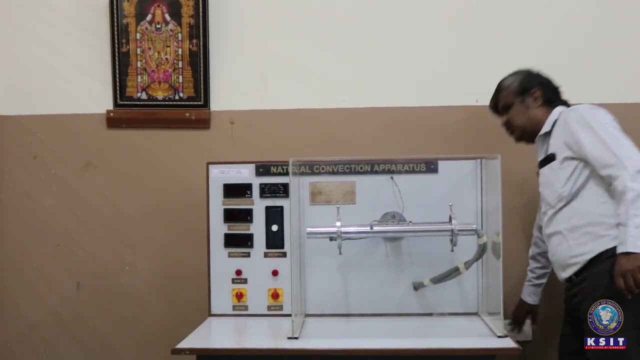 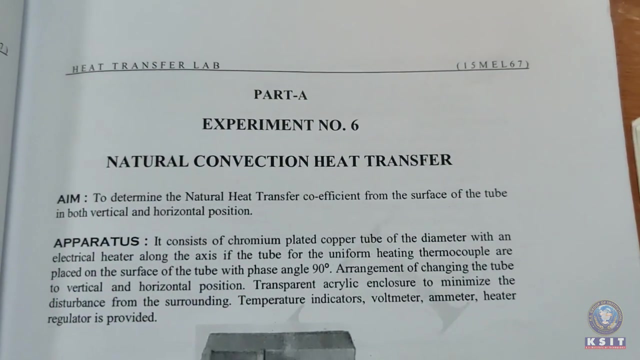 calculations again. we have to switch off this, Switch off the heater, switch off the mains, switch off the console switch and also switch off the mains right. So this: if you do this, you can go back and take the do the calculations part. Now, we will do, we will discuss about how. 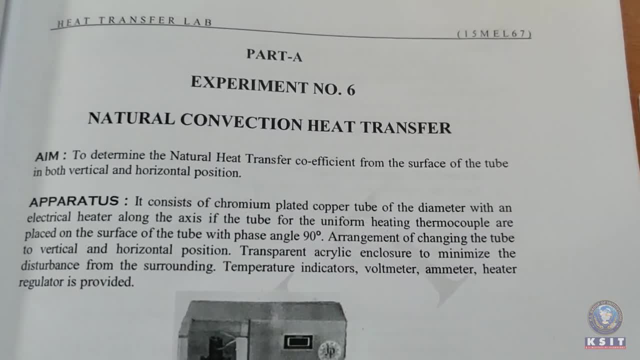 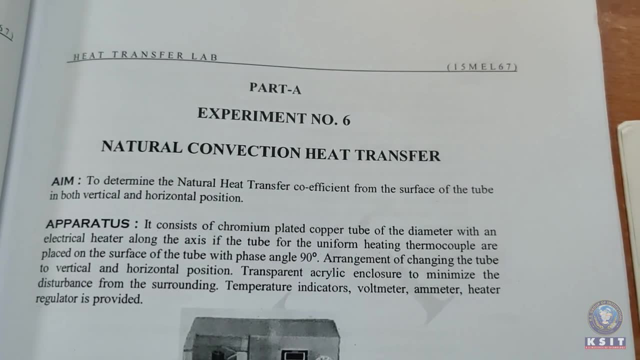 to do the calculations to find the convection heat transfer coefficient in natural convection. right, So you can see the manual. what I am showing now is the natural convection heat transfer. This is from the manual, page number 17,. right So? natural convection heat transfer. 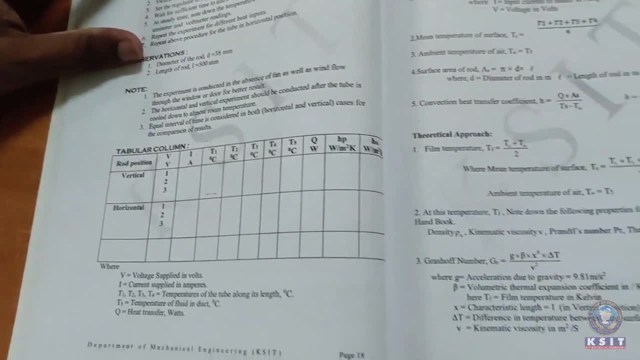 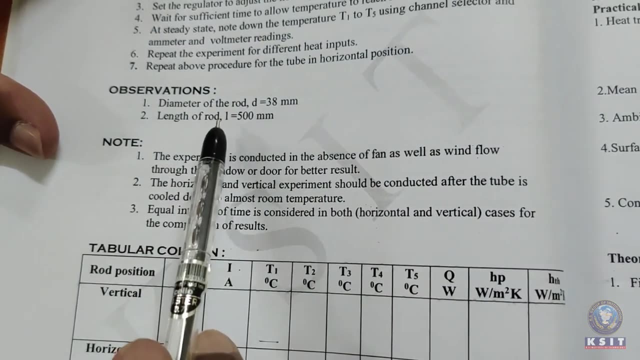 right, So we will go to the next page. This is the tabular column that has been available to us, right? So in the observation you can definitely check the diameter of the rod is 38 mm and length of the rod is 500 mm. 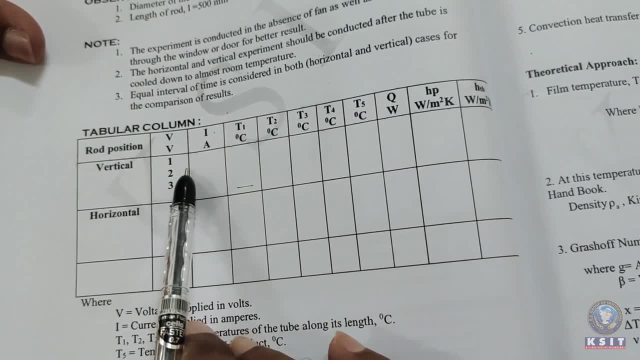 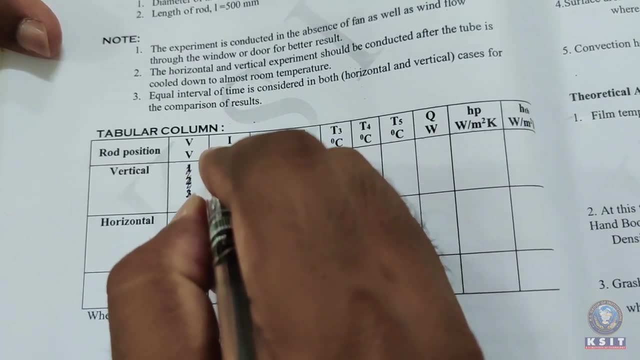 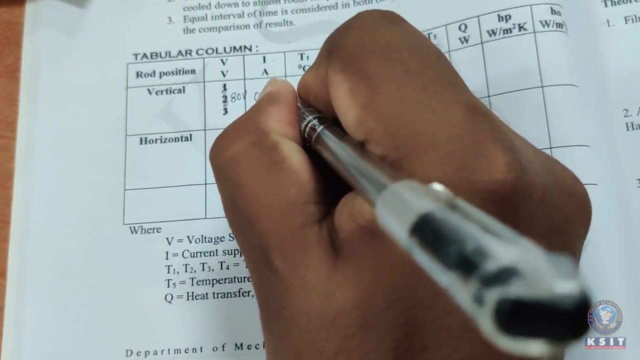 right. Now we will do only the vertical position calculations, right, That is the vertical position: voltage and current. We can write the values. We can have only one trial: the voltage and current values. right, That is 80 volts, for example, and 0.62, right, So do not buy. 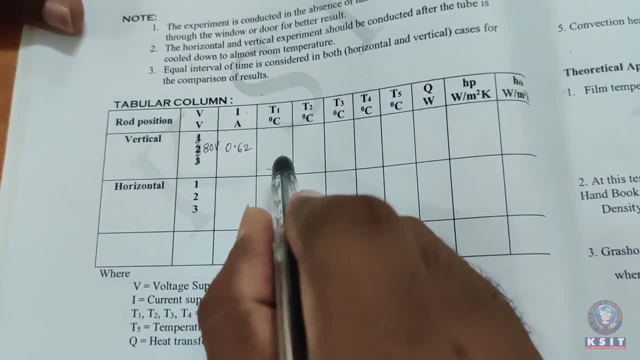 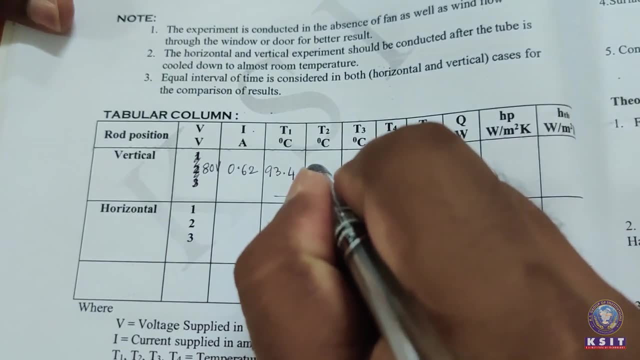 this. You please buy this, So don't buy this, So don't buy this, So don't buy this. So please take the readings and write right. And we have noted the five temperatures, That is. I am giving an example of the temperature values. I am writing the values. That is what we have. 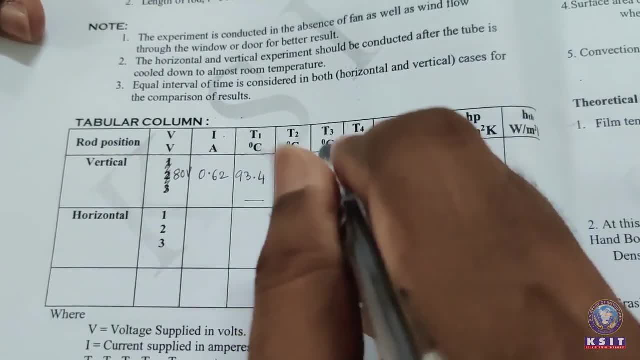 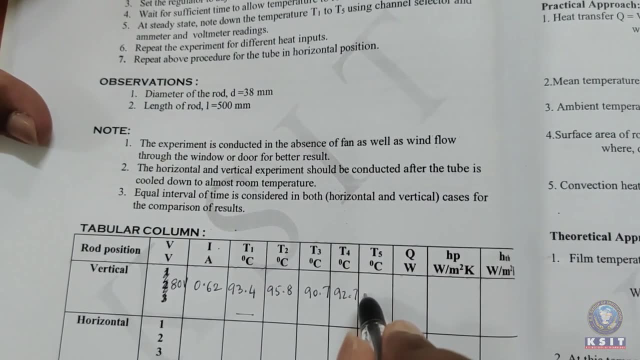 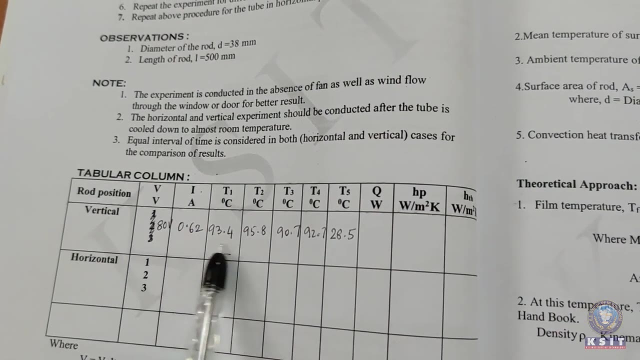 taken the readings from the equipment, That is 93.4,, 95.8,, 90.7,, 92.7.. Then the air temperature, which is quite less definitely 28.5, close to the room temperature right Now. this much is. 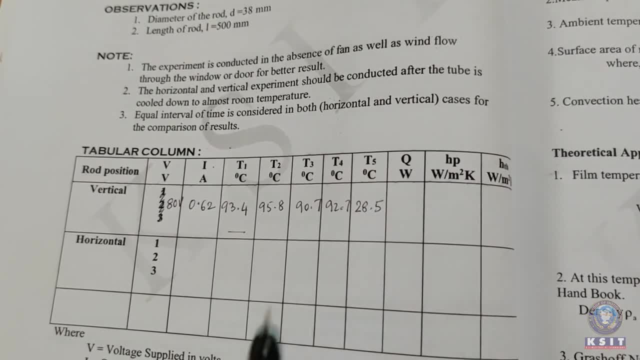 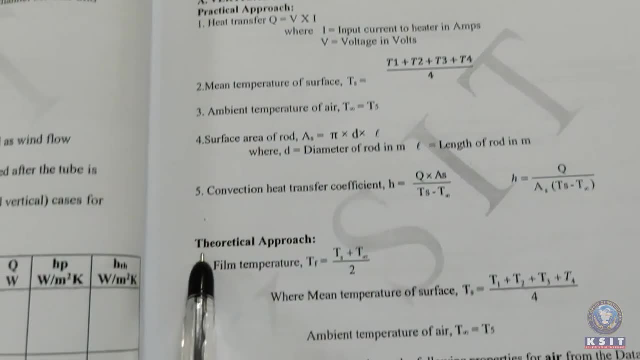 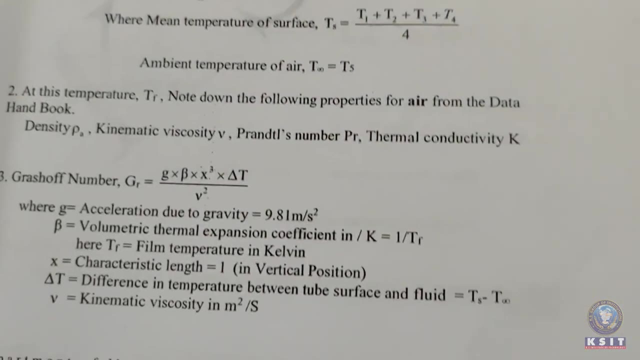 readings that we have taken right. Using these values, we have to find the convection heat transfer coefficient right for practical approach and also the theoretical approach right. So we will go to the calculations pad right, That is page number 19,. right, The keeping the rod in vertical. 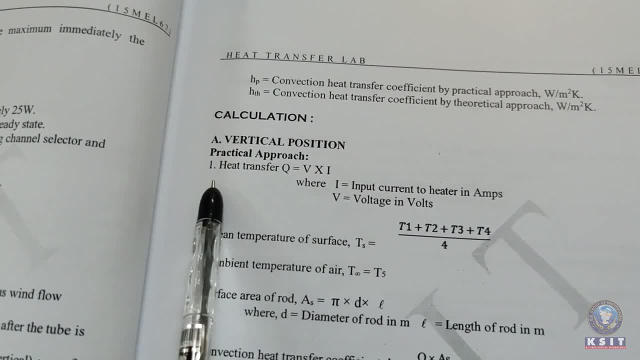 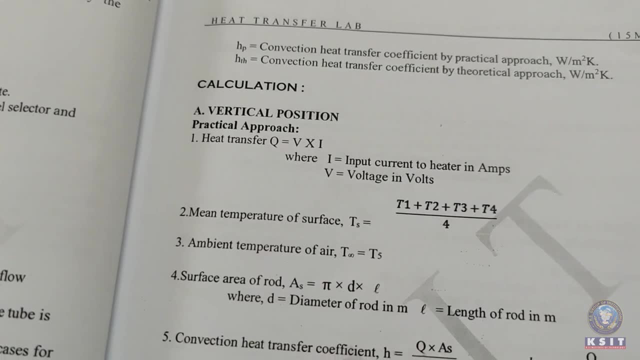 position, practical approach: right. First we have to find how much heat transfer happening, That is, how much taken by the heater, That is, voltage into current. right So, voltage and current. we have the first and the second column in the previous page, right So. 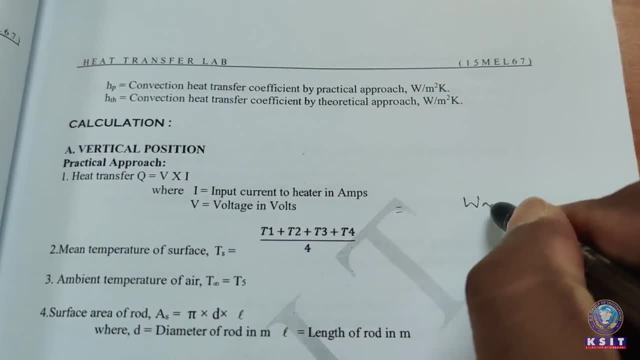 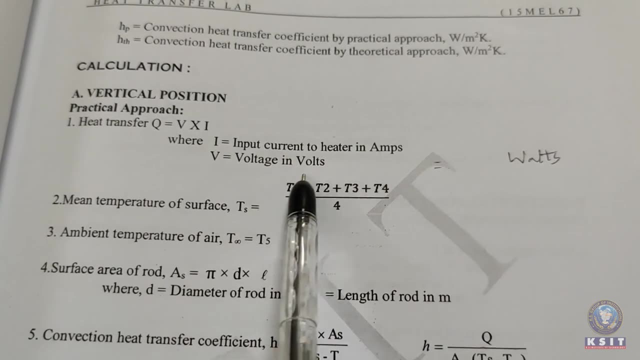 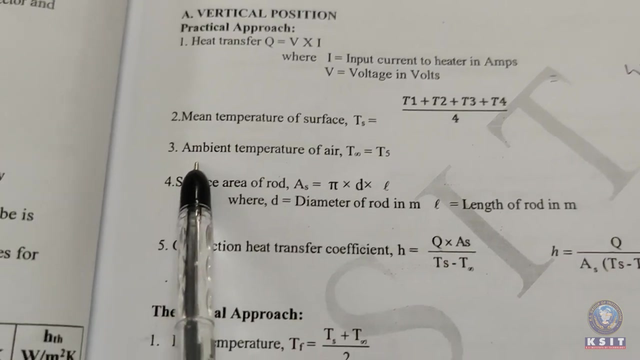 write that value in watts right. Next right mean temperature of the surface. Obviously, the average of four temperature sensors on the surface, T1 plus T2 plus T3 plus T4, divided by 4, is Ts. right Then the ambient air temperature is the air temperature, that is T infinity. 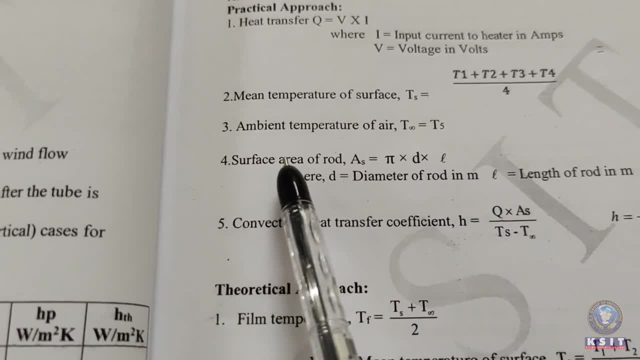 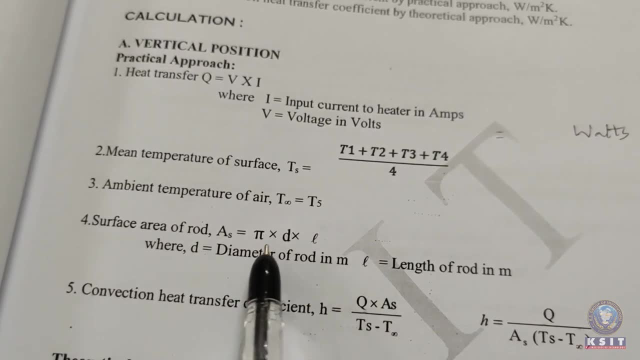 that is definitely the thermocouple T5.. The surface area of the rod, how much area surface area the fluid is touching the rod? That is definitely pi D into the length of the rod right. So pi, DL, pi into 38 mm, into 10, to the power of. 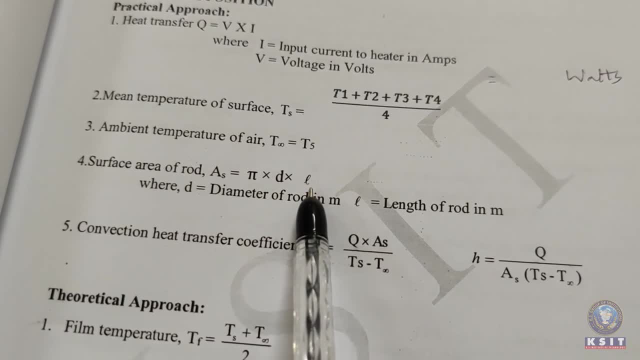 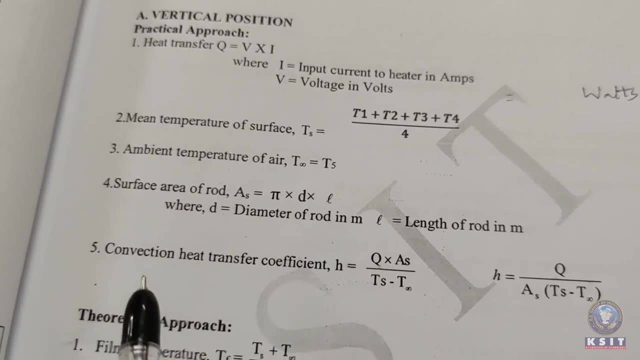 minus 2 meter and 500 into the power of minus, sorry, minus 3 meter right. So I repeat, this diameter and length should be substituted in meter, right, So we get the surface area right. So now we can calculate the convection heat transfer coefficient by simple Newton's law. 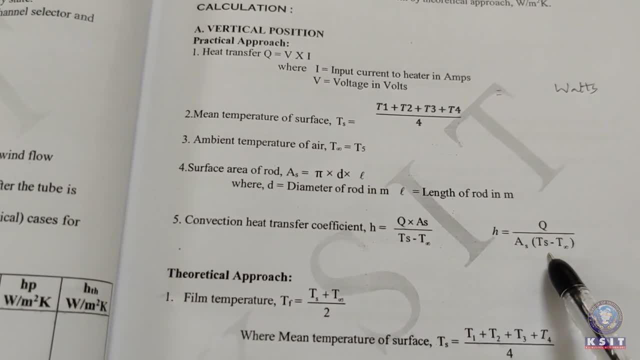 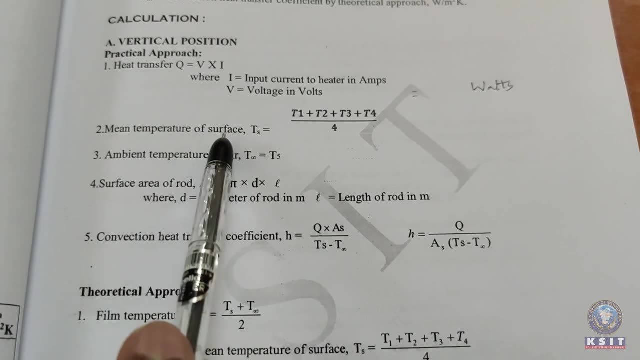 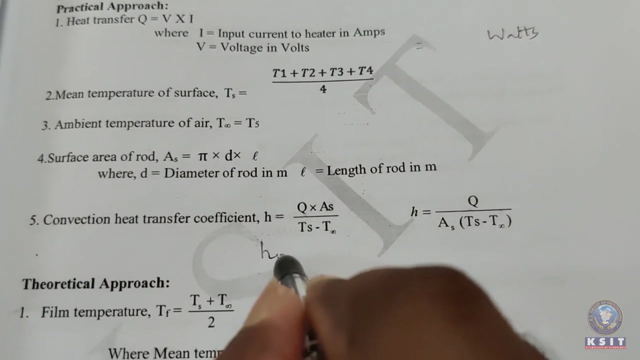 of cooling right. H is equal to Q by As into Ts minus T, infinity Q from the first right surface area from the fourth Ts, second T infinity, third right. So we can get the H vertical position practical value right. So we can get this value and make a note right. So 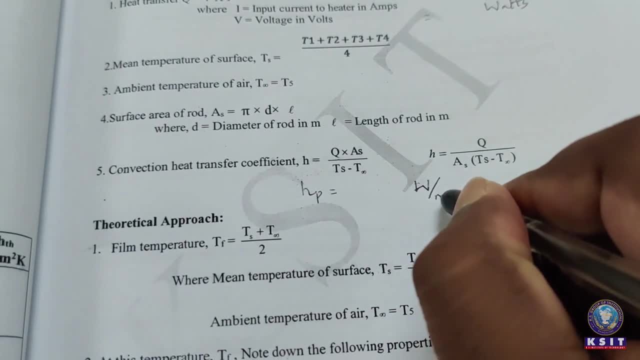 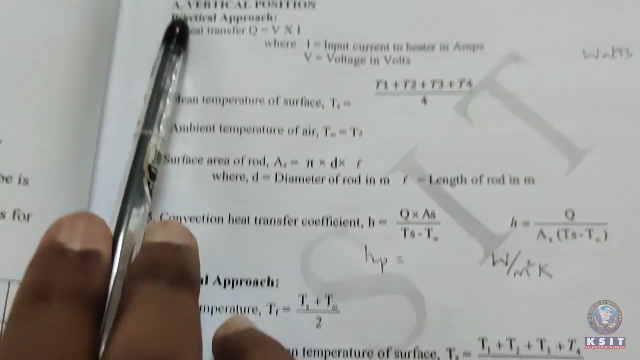 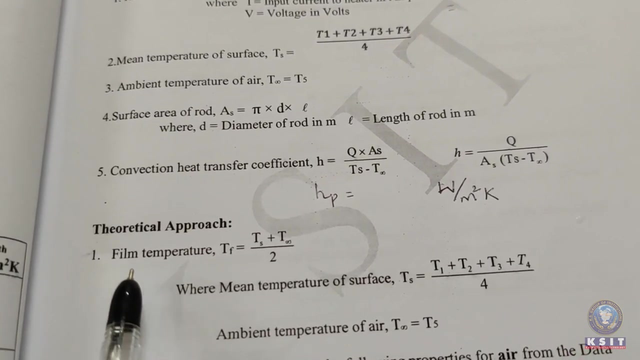 definitely everyone will agree with this. The unit I am writing now is watt per meter square Kelvin. Okay, Rather, the theoretical approach keeping the rod in vertical position. right, Theoretical approach, right. we have to find out the properties of fluid, which is air at this temperature. What is? 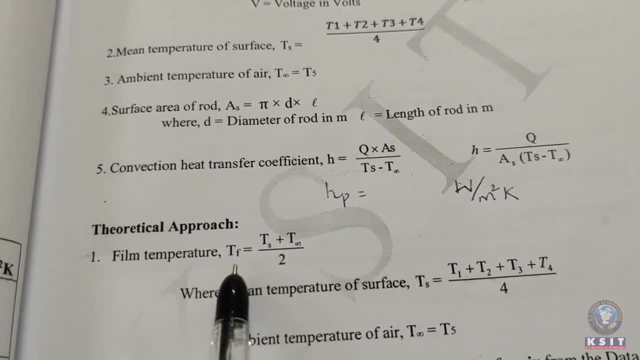 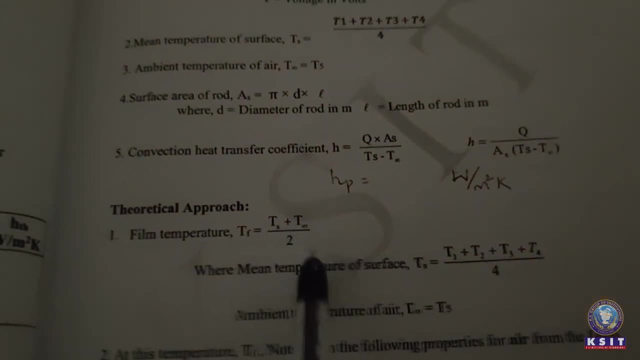 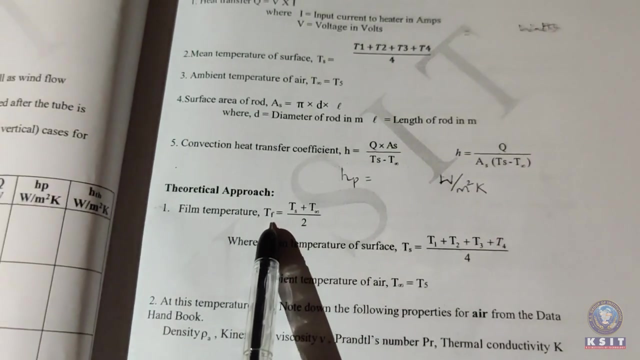 the temperature being called as the film temperature. right, It is an external flow. So Tf is Ts plus T infinity divided by 2,. right, We know Ts and T infinity, right? Take the average of these two and find out the Tf. 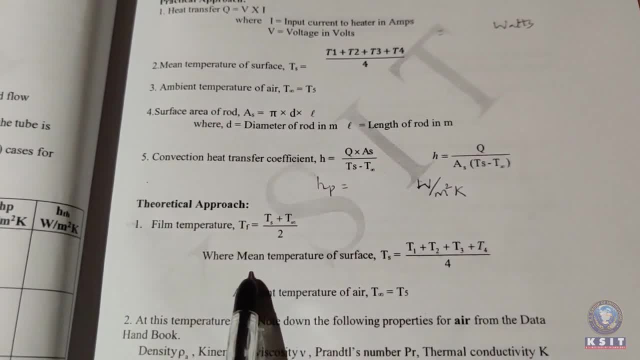 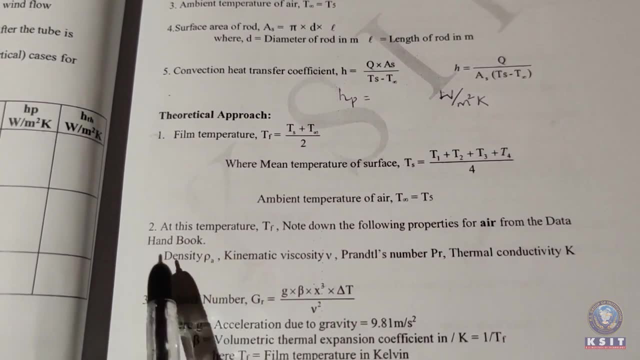 At this temperature, we have to note the properties of air, right? So what are the properties of air? Where we get this? We will definitely get from the data handbook. In the data handbook, page number 34,, right? So please go to the page number 34.. What you can see is the. 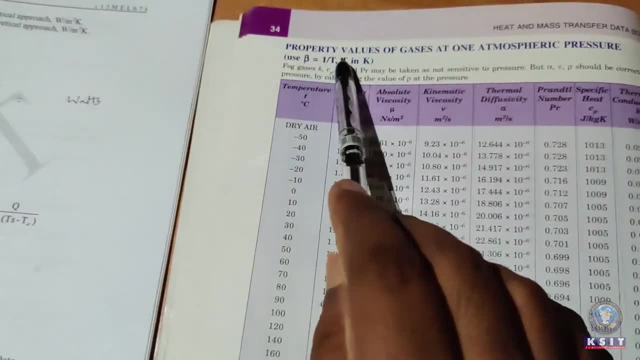 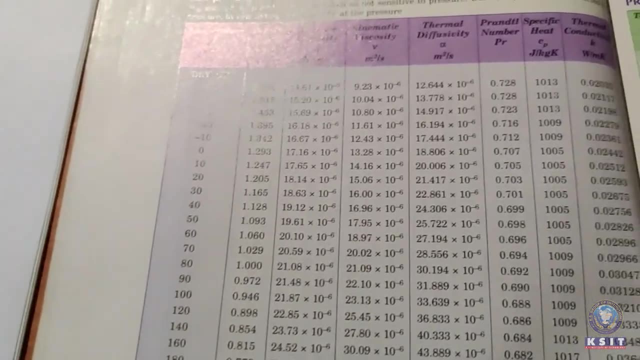 page number 34 in the data handbook, right The property values of gases at one atmospheric pressure, right. So the first column is dry air. In the second page we have the other gases: nitrogen oxygen right carbon monoxide. 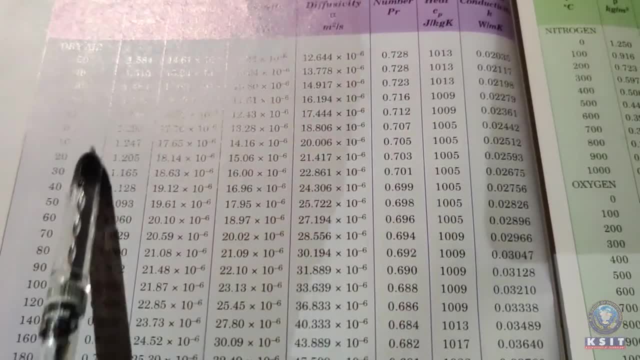 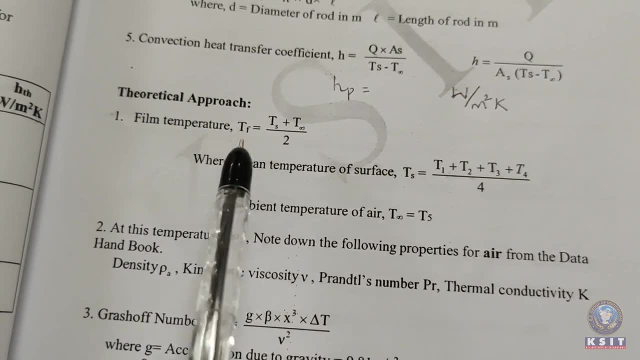 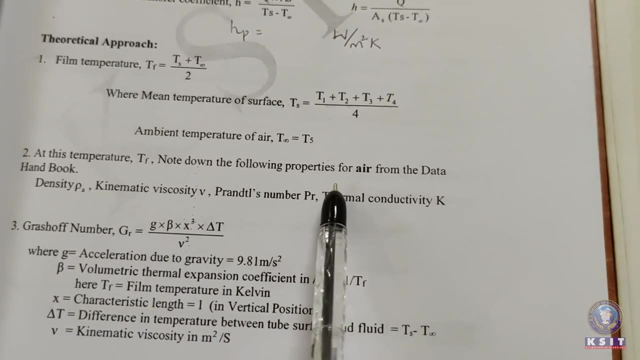 Now we are working only with air, right. So take the properties of air. Suppose it is at 30 degree centigrade At this film temperature, right? we have to find out the properties of air. The fluid is air from the data handbook, right? So where we get from the data handbook? 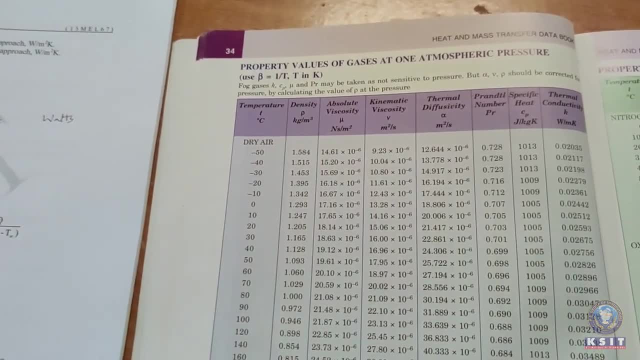 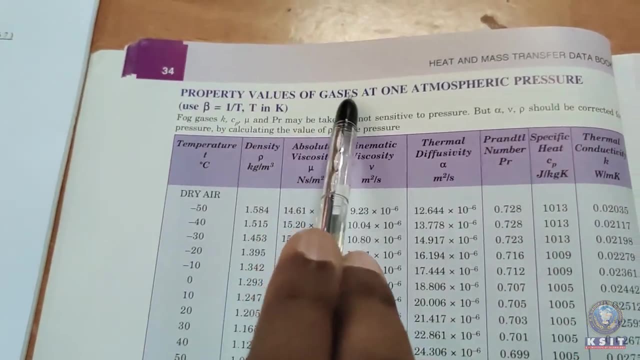 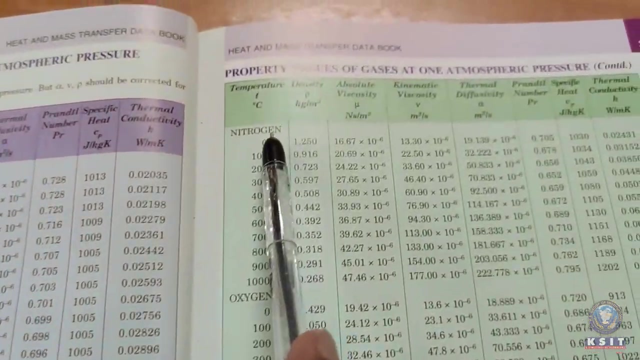 is page number 34 in the data handbook. Now what you can see is the data handbook. Please open the page number 34 in the data handbook right and see the heading property values of gases at one atmospheric pressure. So in this the first column is for dry air. right In the next page we have different gases. 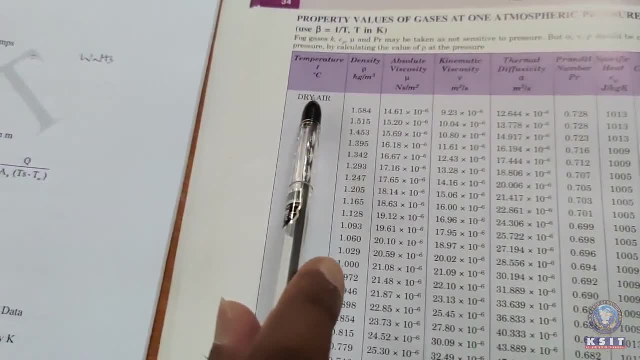 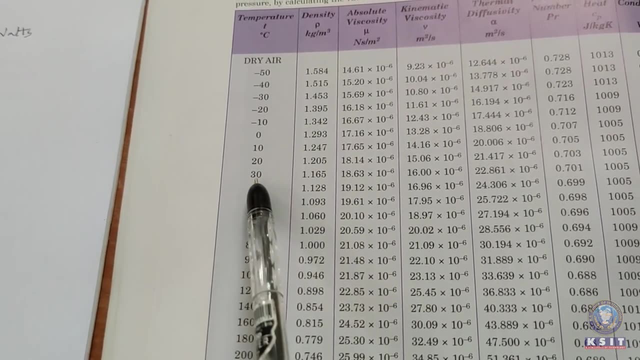 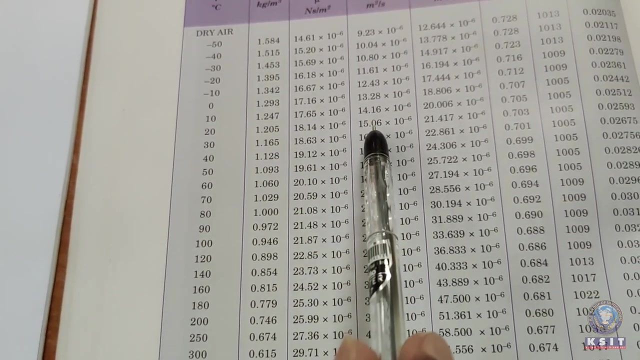 nitrogen oxygen, carbon monoxide. What is required for us is only the air values, right? So suppose it is at 30 degree centigrade. Suppose if we get, suppose if we get Tf as 30 degree centigrade. take the values of density, absolute viscosity, then kinematic viscosity, thermal. 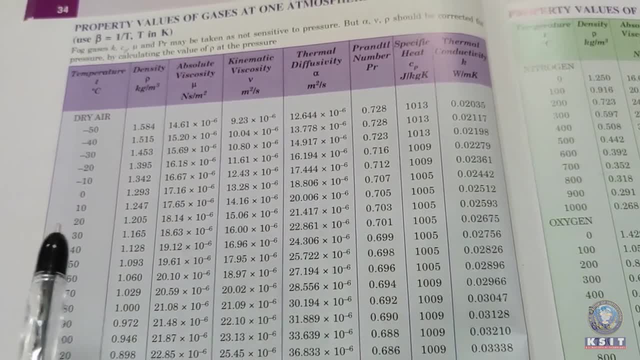 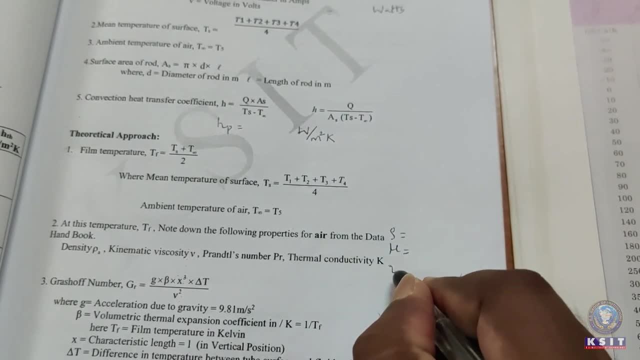 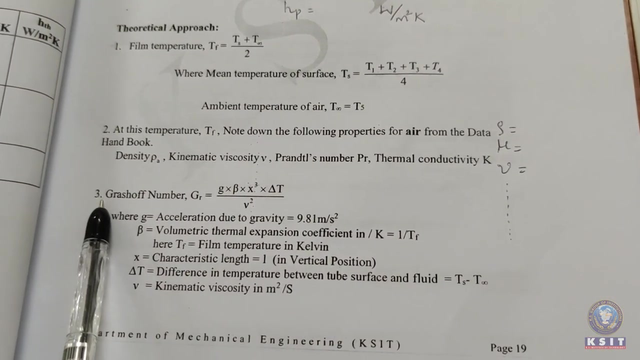 diffusivity, Prandtl's number, specific heat and thermal conductivity: right, And note those values right. Density: right. Next is absolute viscosity, kinematic viscosity, and note all these values for dry air right. Now, the third calculation, what we need to do: 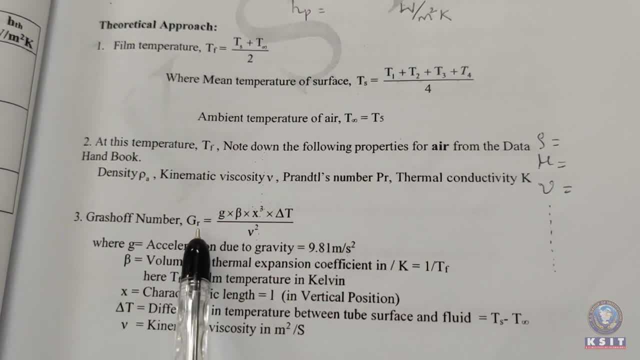 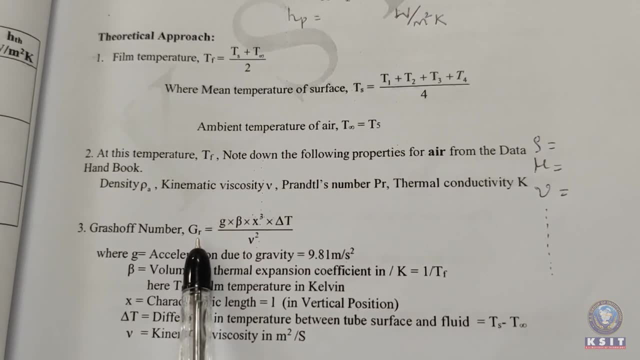 is the crash-off number right. This crash-off number is the parameter, which is a dimensionless parameter, which decides whether the flow is laminar or turbulent. in natural convection, It is synonym to the Reynolds number in force convection right. So 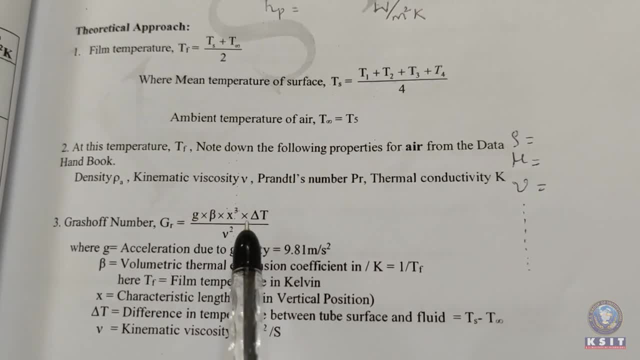 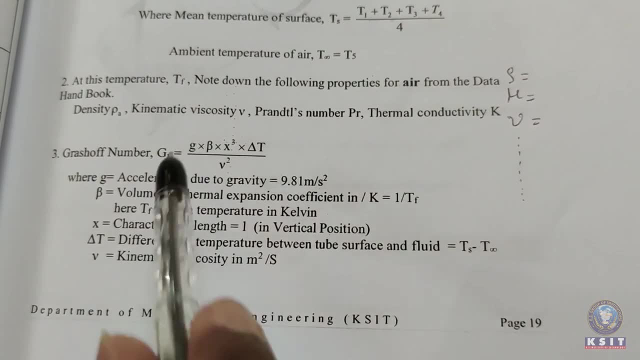 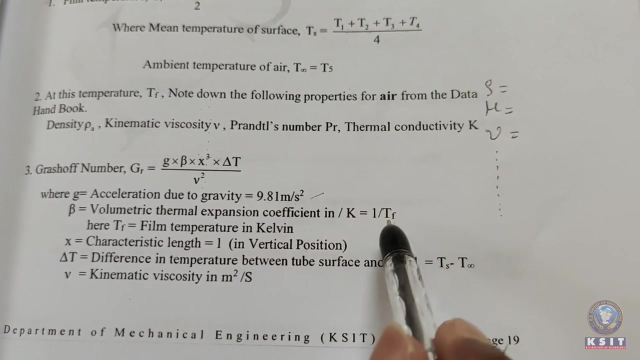 number is given by this formula: G, beta, X, cube, delta, T by kinematic viscosity, square right. So this is very carefully we have to calculate. What is G is 9.81 meter per second square. What is beta is called the volumetric thermal expansion. It is 1 over Tf, but Tf should be substituted in Kelvin. 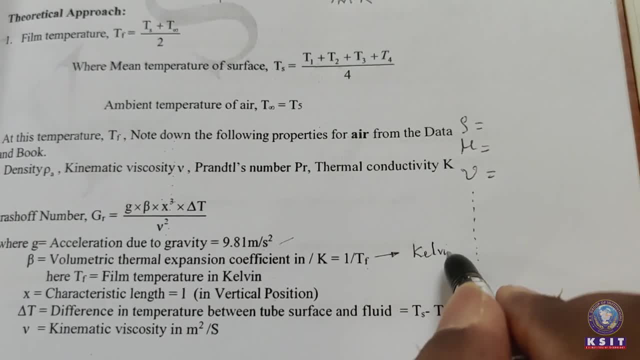 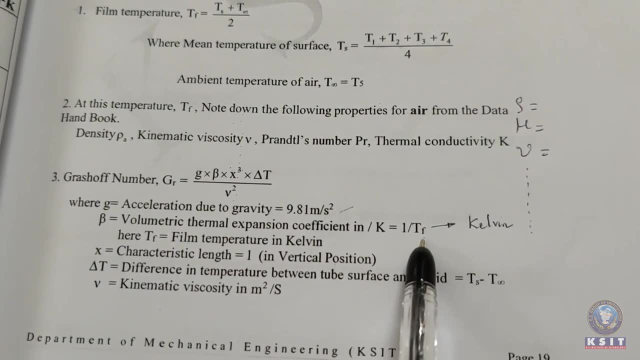 right. I repeat, I am writing again here: Tf- we have to substitute in Kelvin, right Tf. what we got in the previous one is in degree C. right We have to convert into Kelvin and substitute into this equation, right. Next. 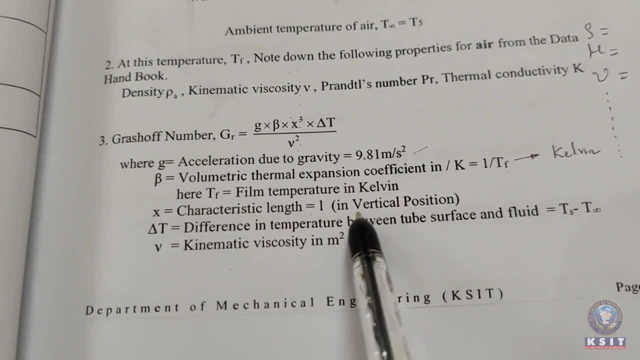 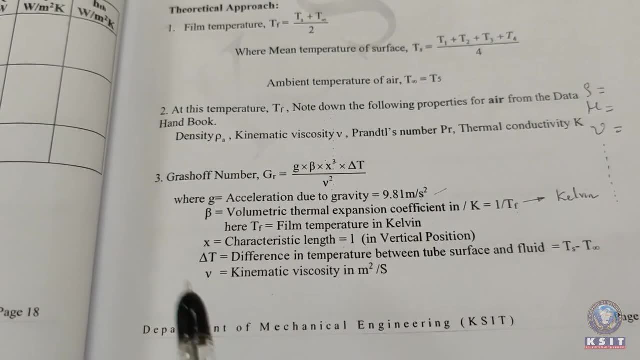 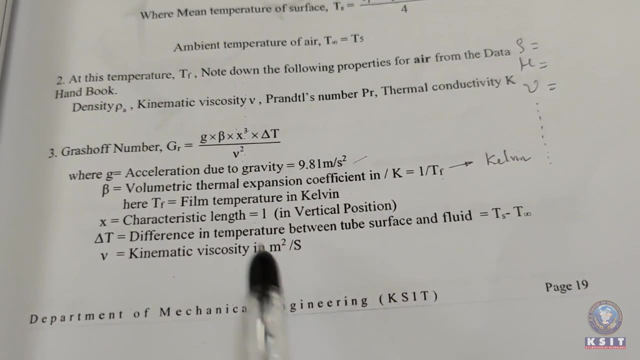 X. X is the characteristic length. Since it is a vertical position, characteristic length is the length of the rod right. That is 500 mm right. Convert into meter right. Next, delta T is Ts minus T, infinity right. We know both the values right. Kinematic viscosity of air is what we got. 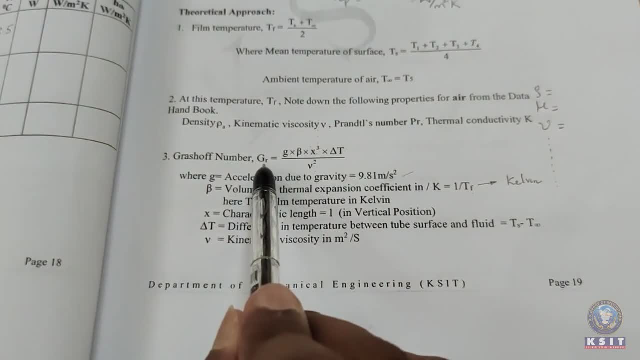 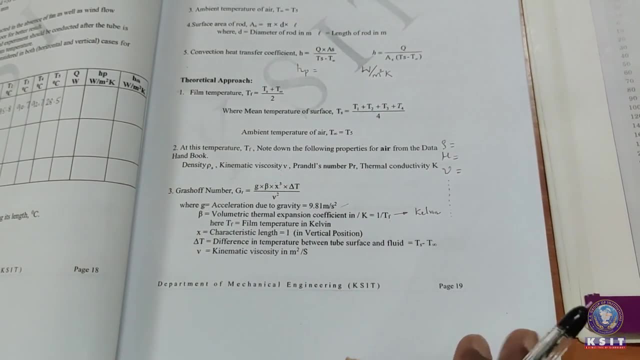 from the dead handbook, right. So, substituting all this, we will get a crash-off number which is dimensionless, which does not have any unit. Now we will go back to the next page, page number 20.. So in the page number 20, right. 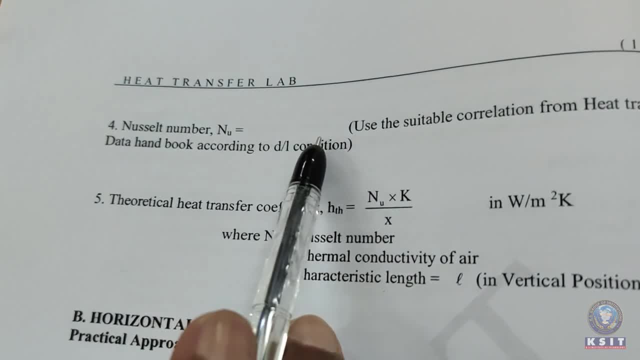 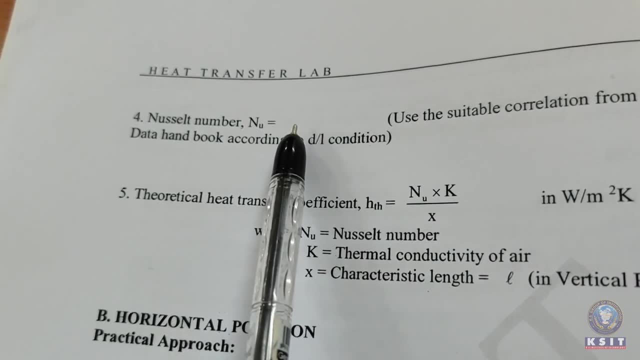 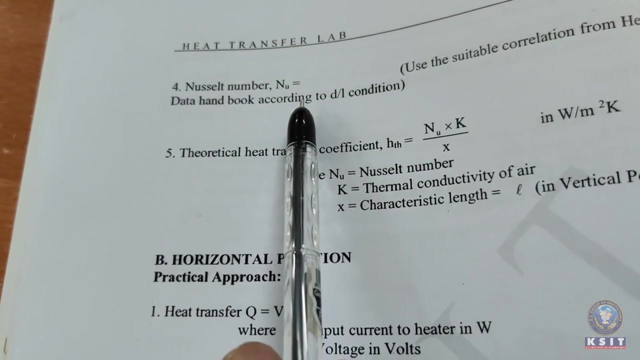 we have to find the Nusselt's number for this condition, right? So we have to use the suitable correlations available in the dead handbook for Nusselt's number and for this situation. right? So we will go back to the dead handbook and find out the suitable Nusselt's. 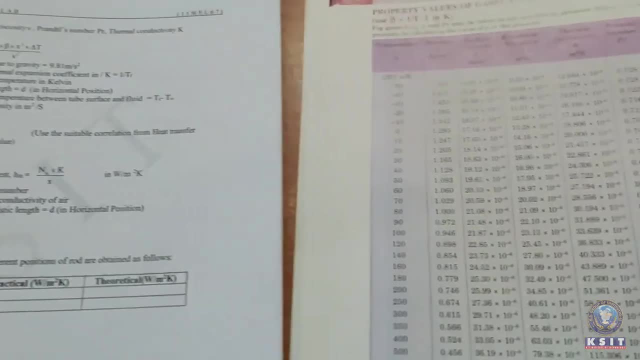 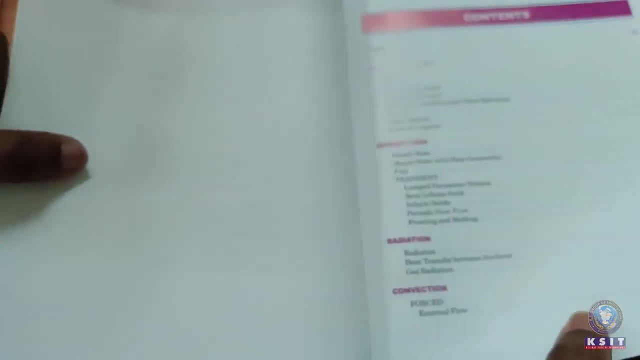 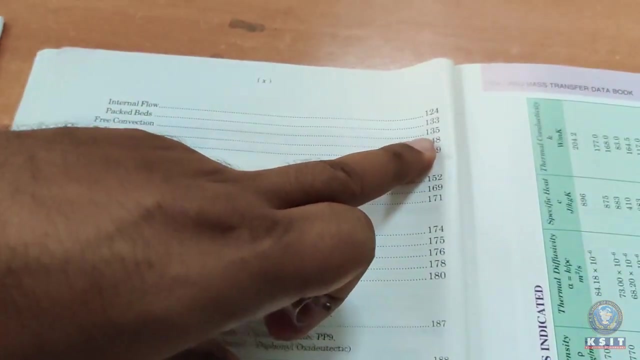 number we have to pick right. so going to the data and book, right. so in the contents page you can check the free convection in the contents page. i'm opening the contents page. you can check the convection, free convection. that's in the page number 135 right now, the free convection. what? 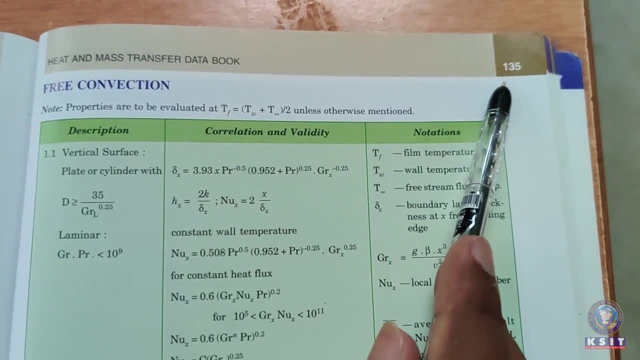 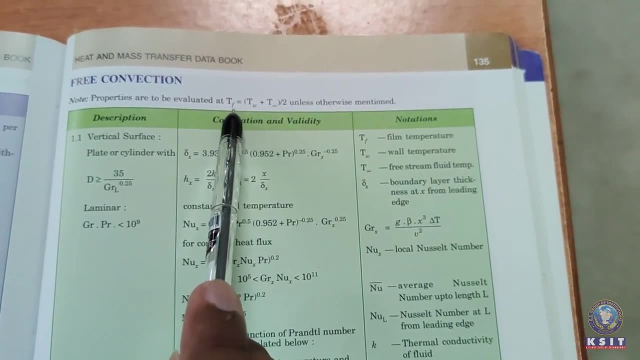 we can see. this is from the data and book right, page number 134 in the data, 135 in the data and book- please open the page number 135- and the properties are to be evaluated at dm right. that is a film temperature. this is the temperature, what we have noted right. so vertical surface. 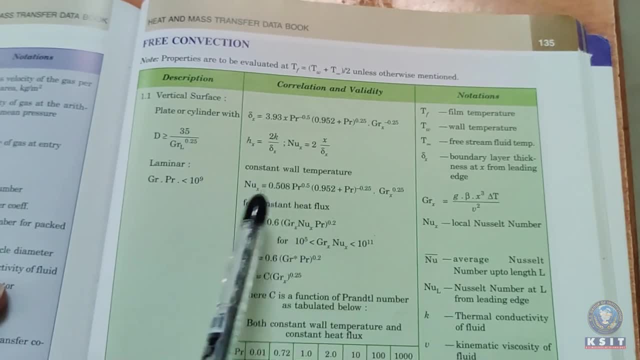 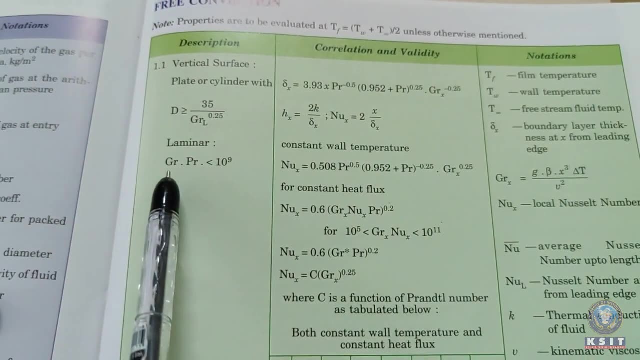 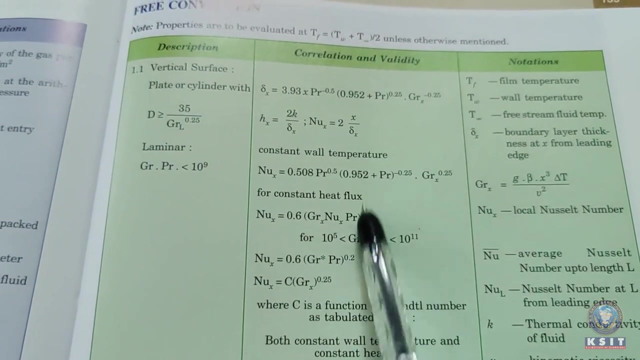 is what we are supposed to do right in this. these correlations are suitable for grpr less than 10 to the power of 9. that is laminar right. so find out the product of grpr. crash of number into pandas: number right if it is 10 to the power. if less than 10 to the power of 9, use this correlation. 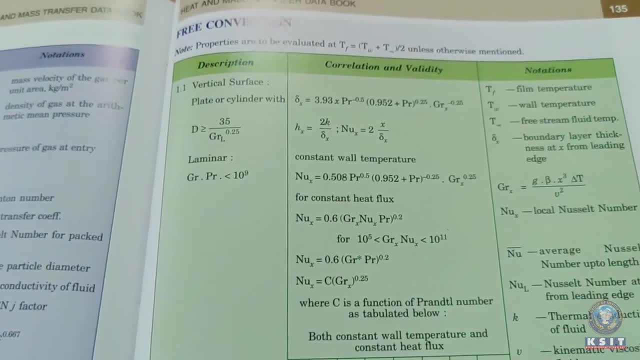 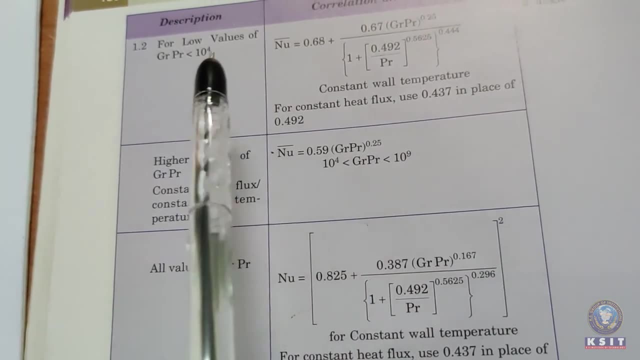 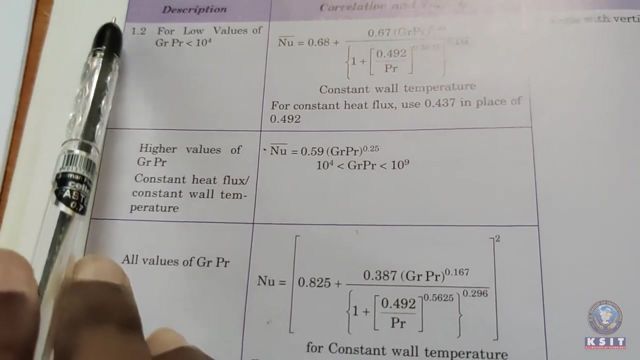 right now, from the previous experience, what we get, what we have right, grpr will be greater than 10 to the power of uh. grpr will be a higher value, will be a higher value. so we can use this correlation- higher values of grpr right and in the page number 136 right. so we will definitely use this. nazar's number is 0.59. 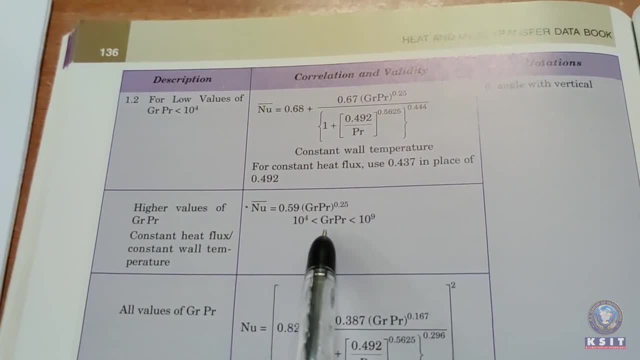 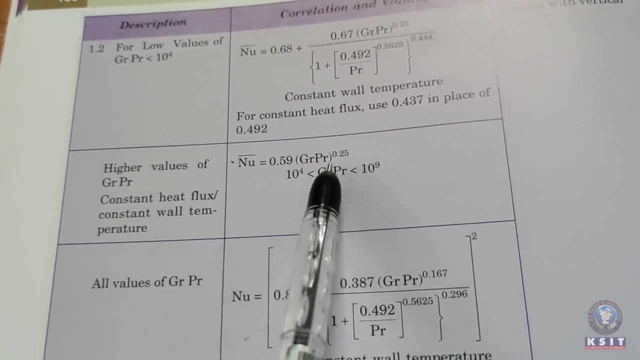 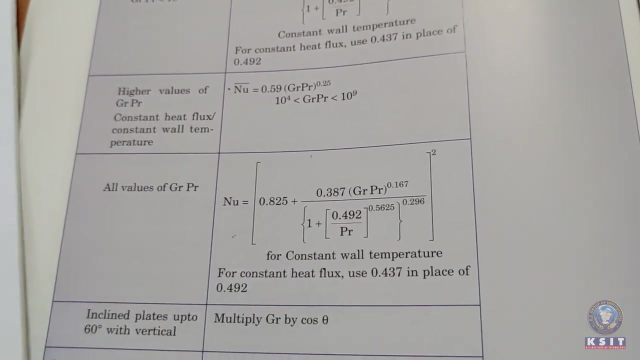 grpr to the power of 0.25. please check whether the grpr will be fitting into this range right, so use this correlation: genu is 0.59 grpr to the power of 0.25- right. come back to the manual right. substitute the values. 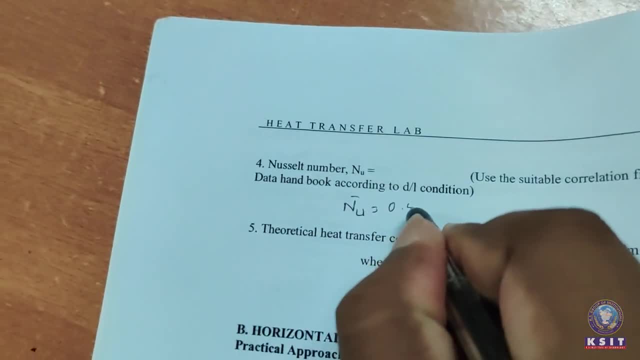 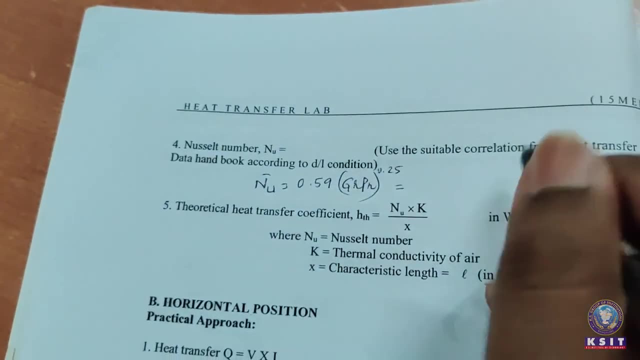 for that, for that equation, nu bar 0.59, 0.59 grpr to the power of 0.25, substitute the values of grpr and you will get a nazar's number value right. so using this nazar's number value, we can find out: 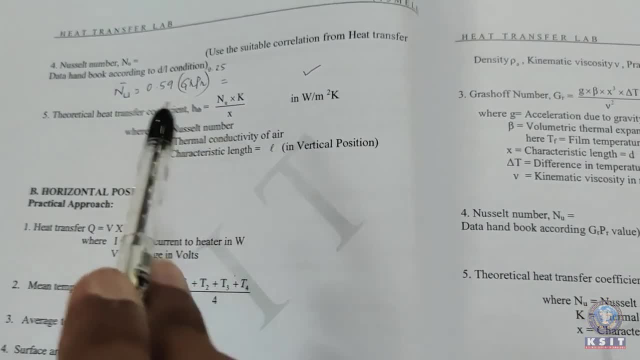 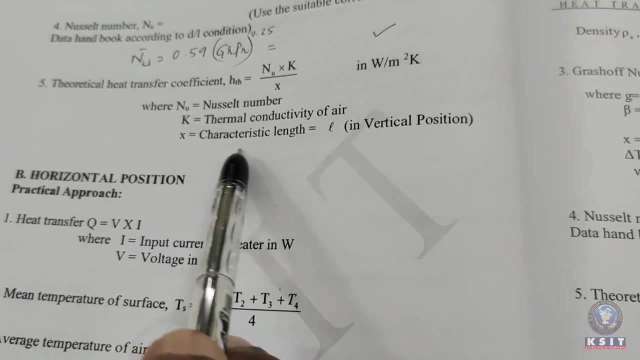 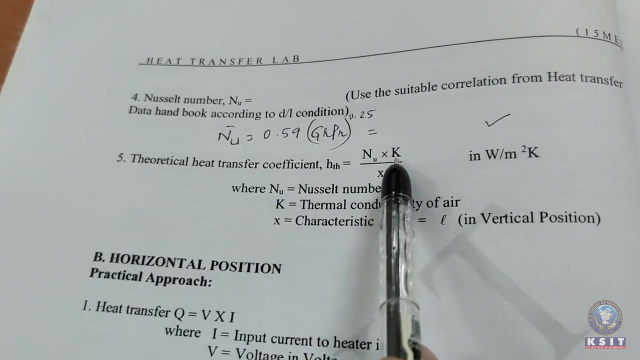 the theoretical heat transfer coefficient h. h theoretical is given by this, nu, k by x, right, x. we are written here because x, the characteristic length for the vertical position, is the length length of the rod right. so nu from the previous previous previous value. k is the thermal conductivity of air, that is, from the property. 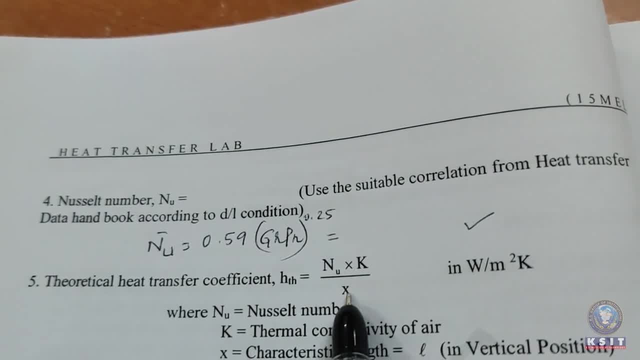 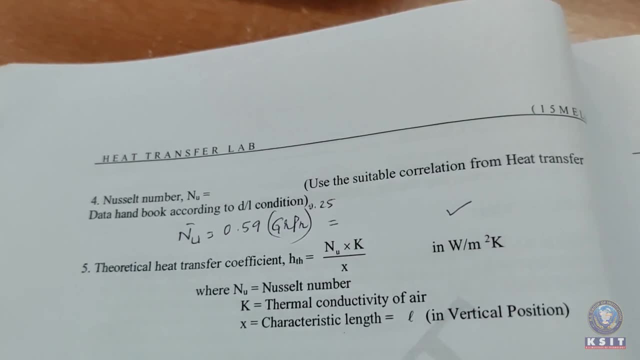 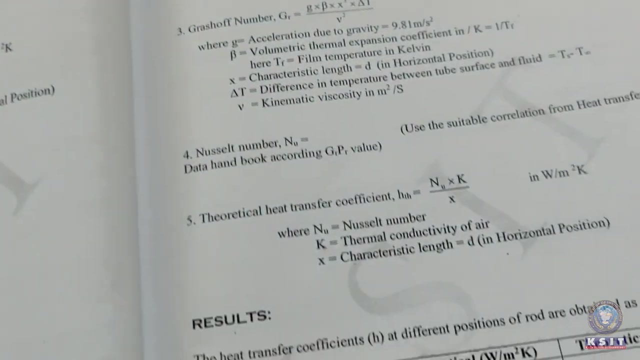 table and x is the length of the rod that we know right. so using this we can find out h theoretical, right. so please remember the h, h practical and h theoretical value, keeping the rod in vertical position, and go to the results and fill these two values. what we are filling now is vertical position, h practical value hp. 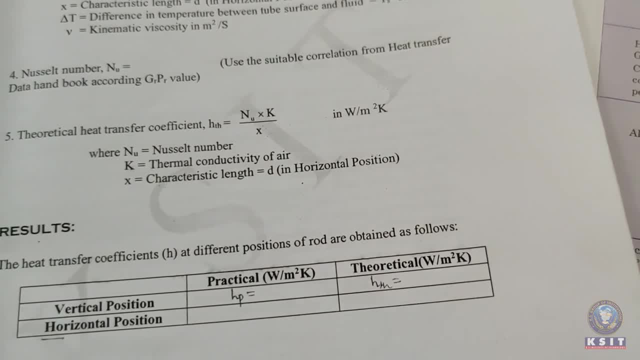 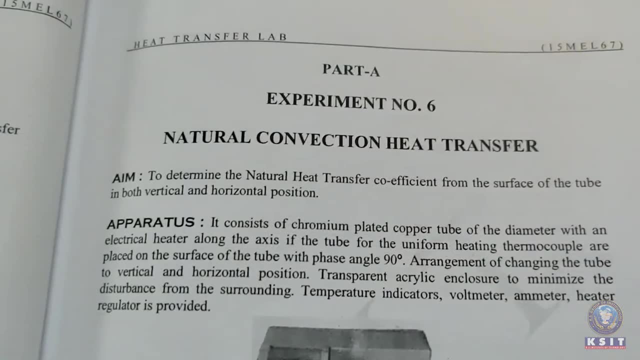 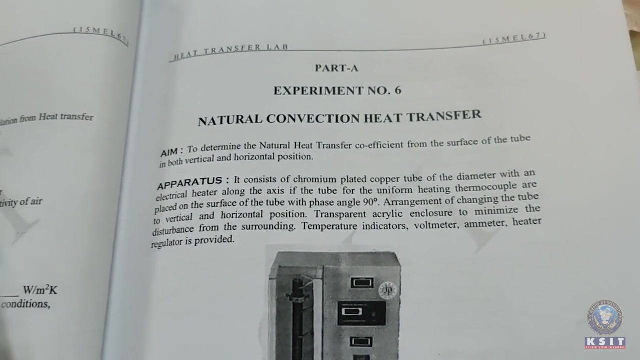 and h theoretical value HE. so this much is the calculations to be done for vertical position. we will start now discussing discussion about the calculation part for natural conventional transfer, when the rod is present, into a vertical position. so till then we are off to a good run. it transferred when the rod is kept in horizontal position, right. so the same page, number 17, right. 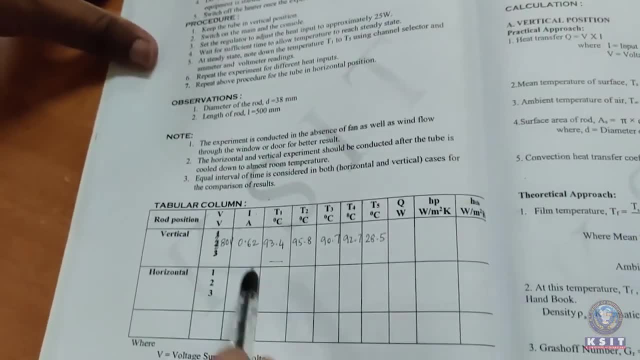 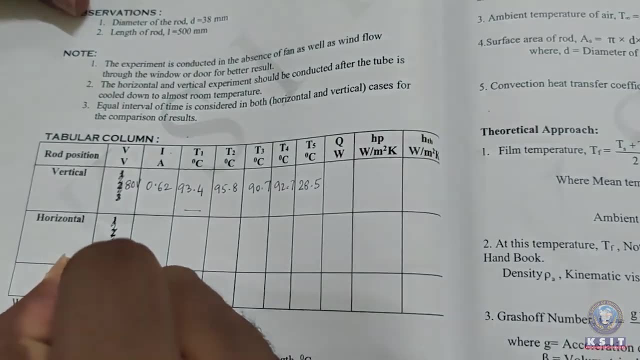 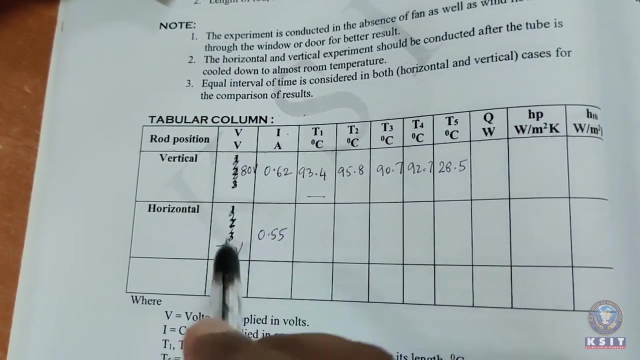 so i'm going to the natural convection and in the tabular column i am now i am writing the values, what we have taken for horizontal position right, first column, the 70 volts right, followed by the current of 0.55 amps right. this is for horizontal position. everyone can definitely check it right. 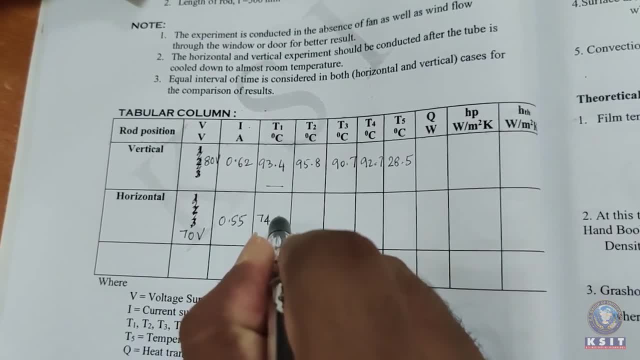 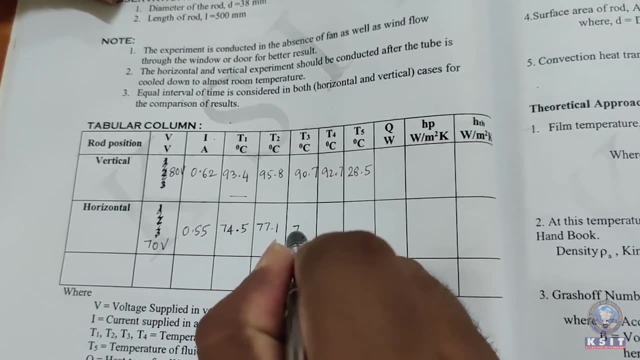 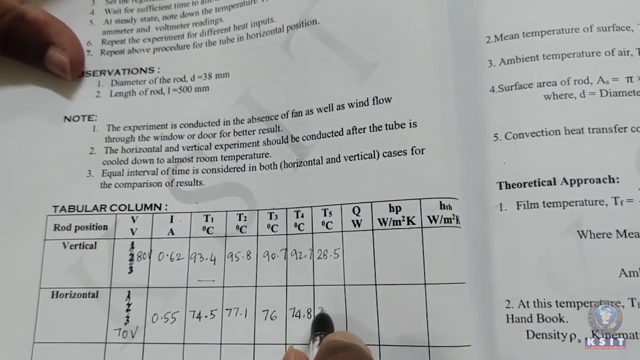 then i'm noting the temperatures on the surfaces, that is t1, 74.5. next, 77.1 is t2, 76 t3. 74.8 is t4. right, and now the air temperature which is closer to the ambient, that is 27.7. right, so the four. 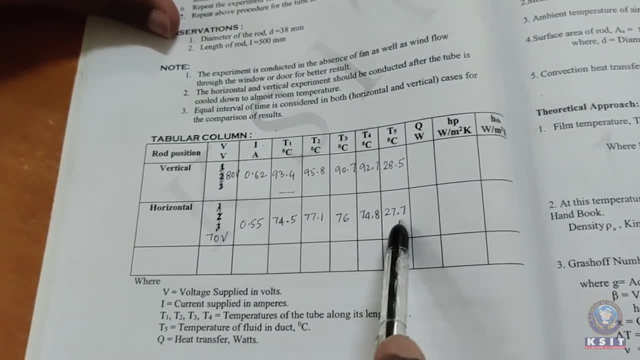 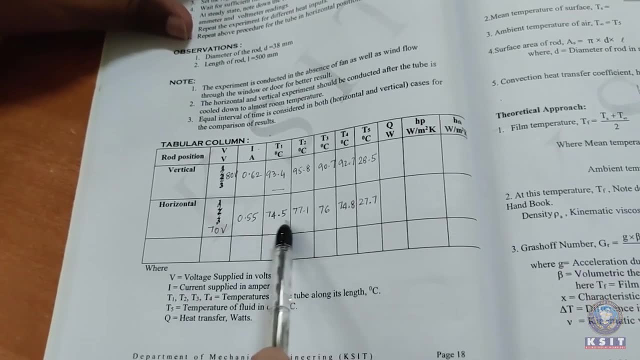 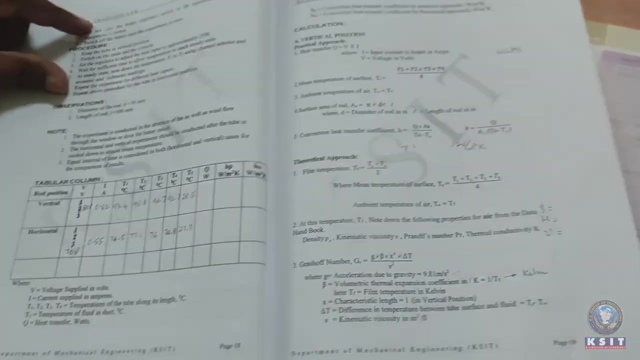 temperatures are this and this is the air temperature. i am giving only this as an idea about the temperature values, right? so whatever the readings you get, you have to enter those values on these columns. right the calculations pad. you can go to the page number 20. that is been uh in the manual, that is b. 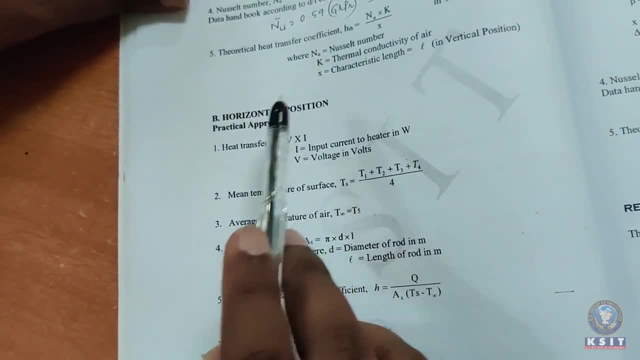 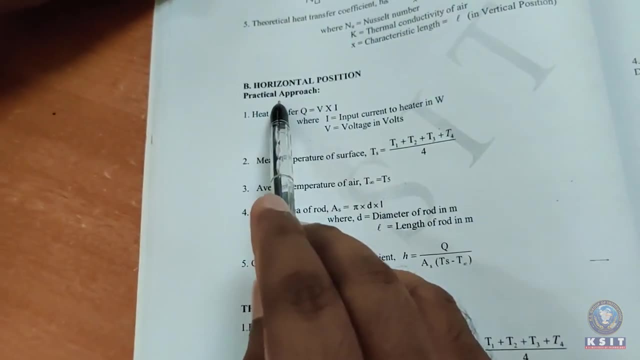 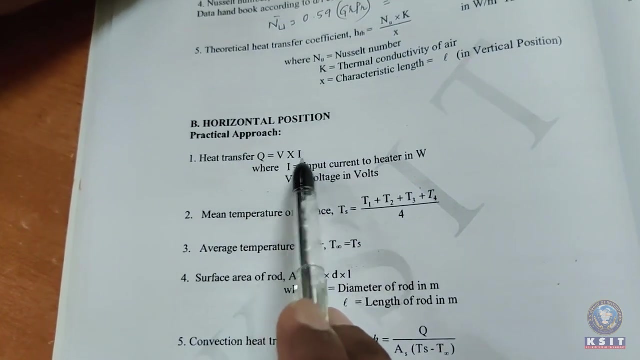 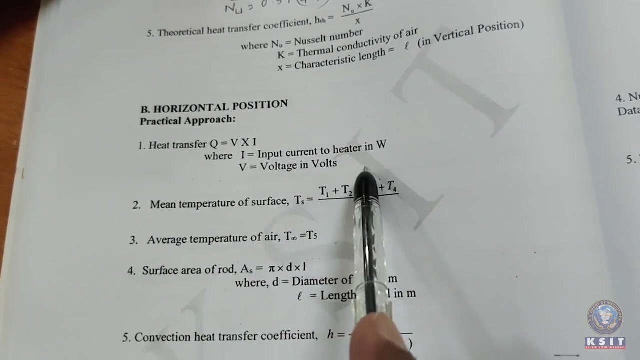 horizontal position, right horizontal position. we have to calculate the h value by practical approach and also by theoretical approach. first we'll do by practical approach. the first one is similar, is is quite obvious: the heat transfer is voltage into current for horizontal, uh, horizontal position. whatever the voltage and current, we got right here right. then surface temperature is the average of four. 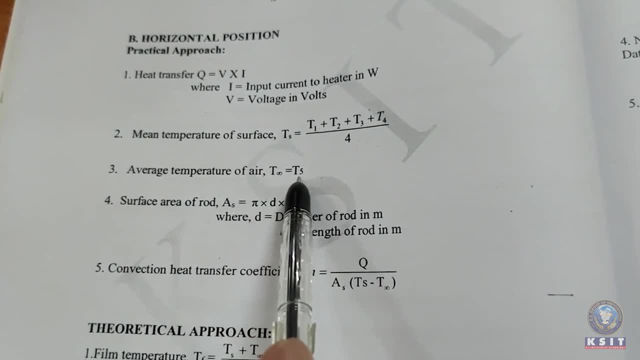 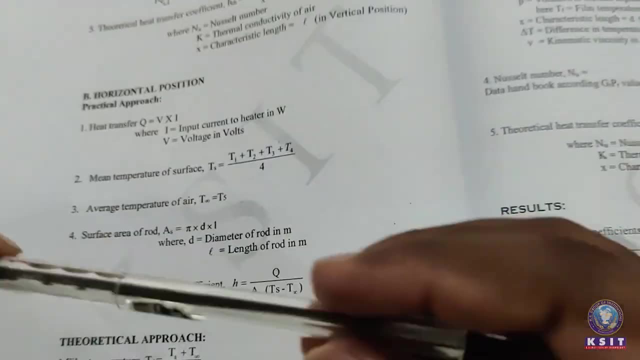 temperatures on the surface. the temperature of the air is the ambient temperature, that is, t. infinity is equal to t5. right now, the surface area, the surface area when it's kept in horizontal position, is the same. surface area, right so pi, dl, right so diameter, length of the rod is same. 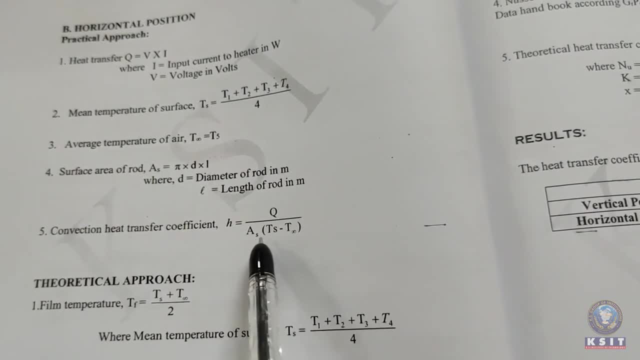 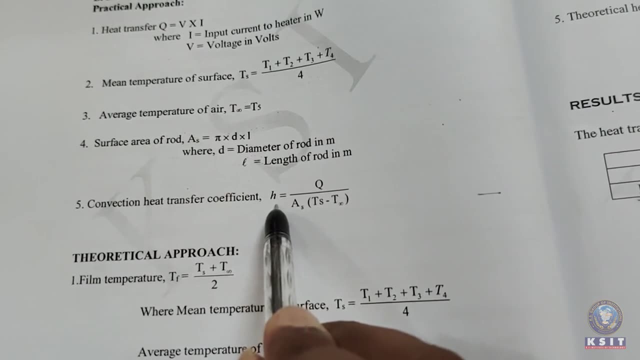 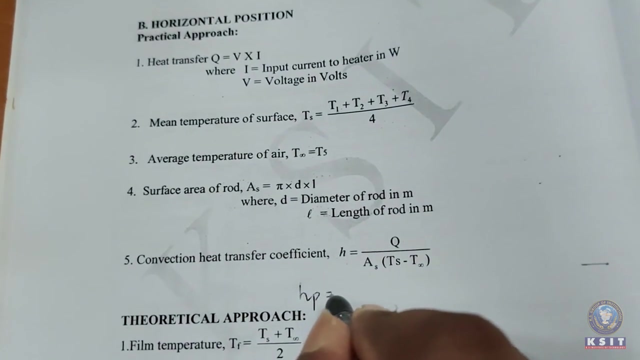 right. so we can find out: the h value q by a s is equal to t s minus t, infinity right. the formula is say: but the value of h we get different when, when it's been kept in horizontal position, because the temperatures will be different. right now, this much is the h practical value of the rod when it's 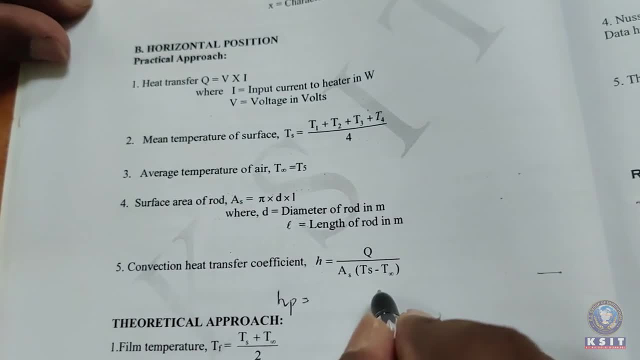 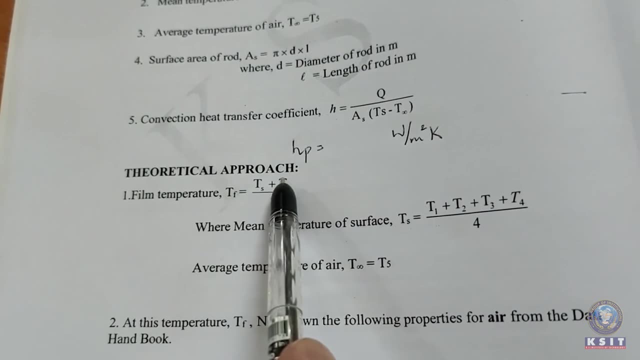 kept in horizontal position. right, so we can write the value, and definitely the unit is watt per meter square kelvin. the theoretical approach is the same, but we can write the value of the rod as the pressure to find out the value of h. right, so again the film temperature at which we have to take the 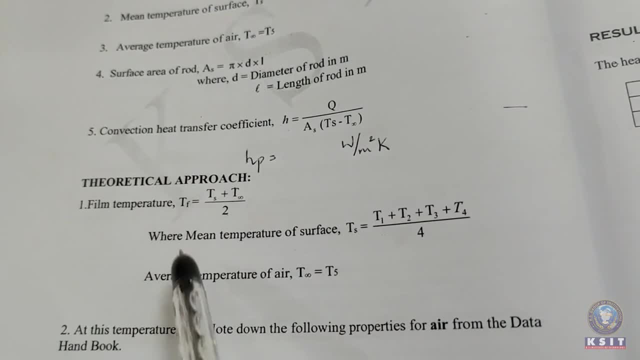 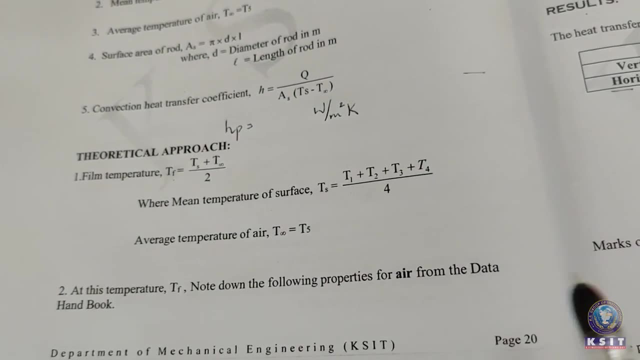 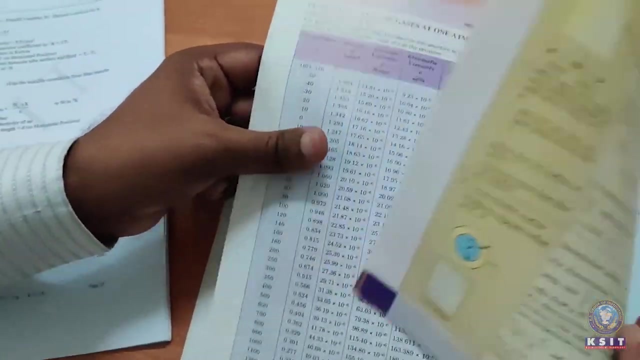 properties of air is ts plus infinity divided by 2, right. so at this, at this temperature, find out the properties of air from the data handbook. the data handbook, the same page number, same page, number 34- i'm sorry for it, page number 34- and you can see the properties of. 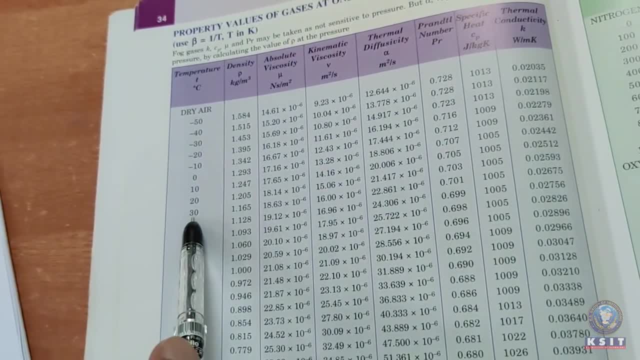 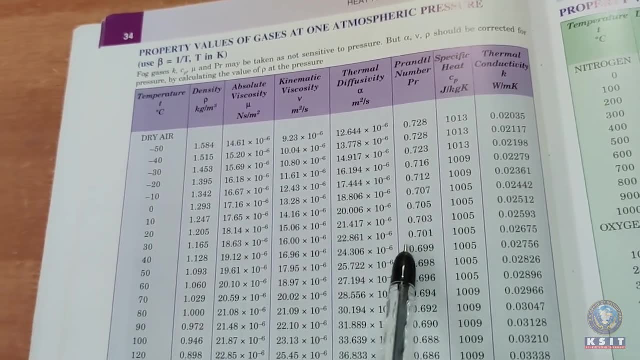 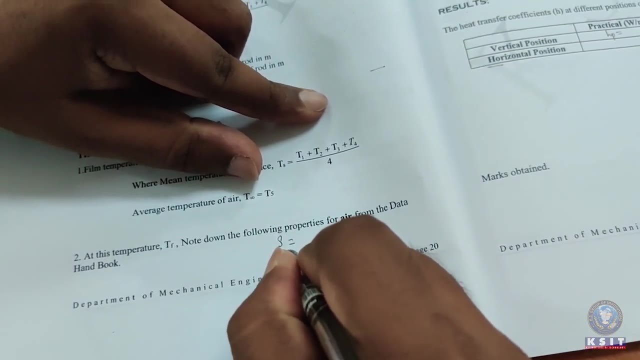 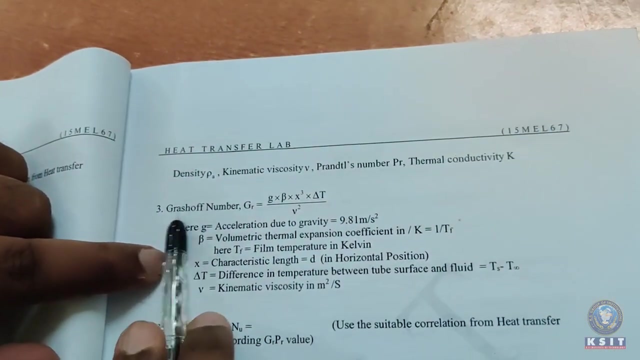 gases. that's a dry air, suppose if we get for, say, 30 degree centigrade again. note on note the density, viscosity, thermal conductivity, specific heat, brandless number for air. i am quite obviously we need to write the values here: rho, mu, nu, cp, values of air right. so now the third part. we 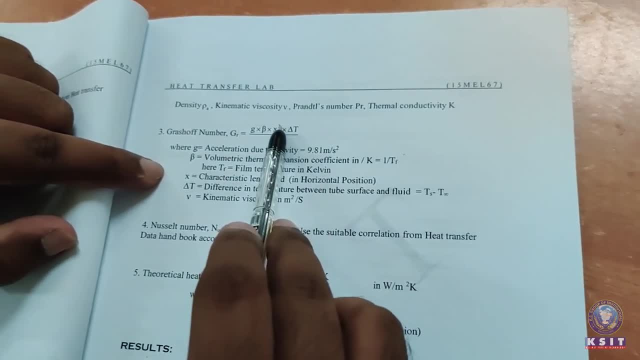 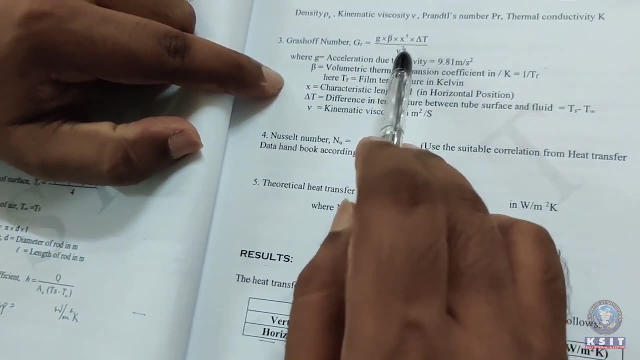 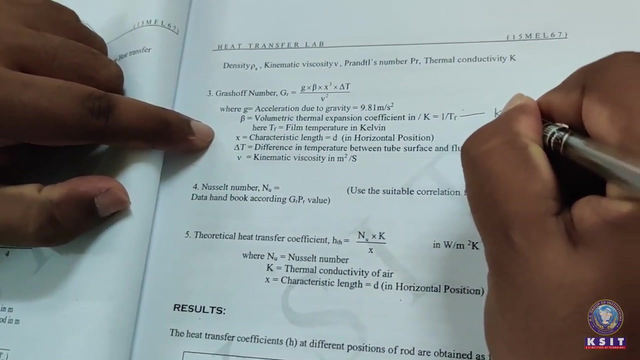 have to find out the crash of number when it's kept in horizontal position right. the crash of number number when it's kept in horizontal position is. the formula is same: g, beta x, cube delta t by kinematic viscosity square right: g 9.81 beta 1 over tf. tf should be in kelvin right, then characteristic. 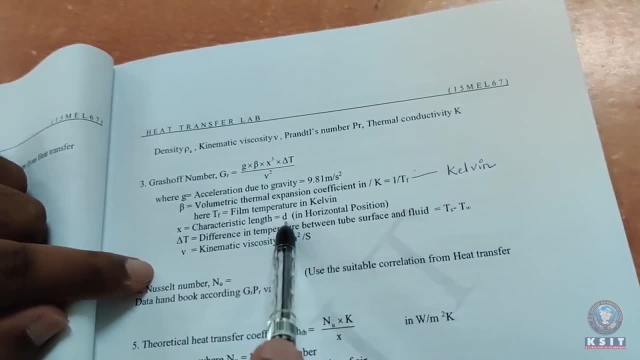 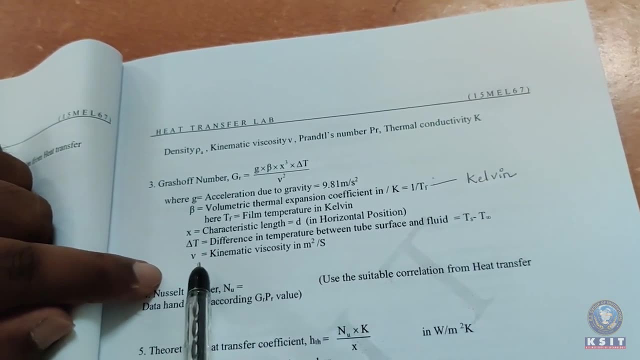 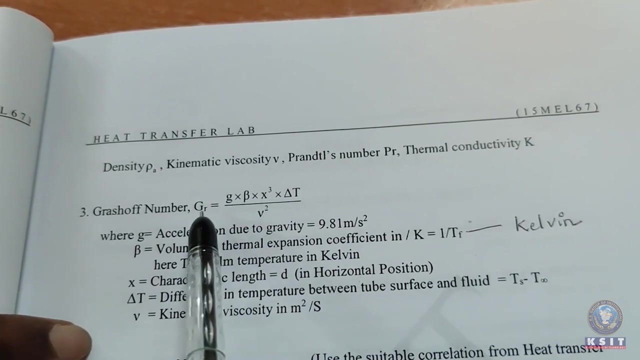 length for horizontal position is the diameter, not the length of the rod right. then delta t is difference in temperature, ts minus t. infinity. then kinematic viscosity of the air. we are taken, we can take, you can definitely get from the property tables right. so using this, find out the crash of. 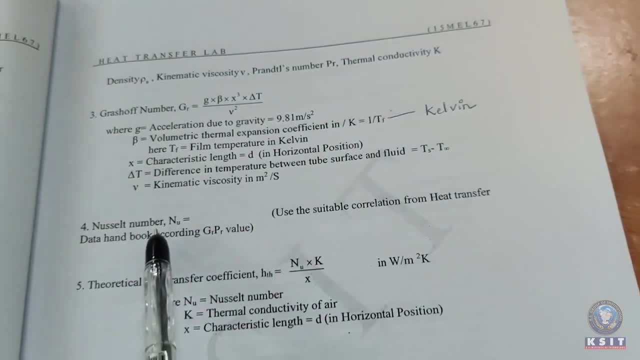 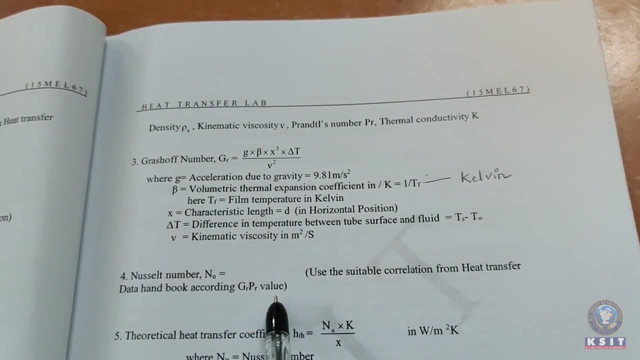 number. right after finding the crash of number, we have to find out the nuzzle's number, nuzzle's number. we have to find the suitable correlation for horizontal position from the data handbook. so go to the data handbook right. go to the data handbook, page number 135. you can check free. 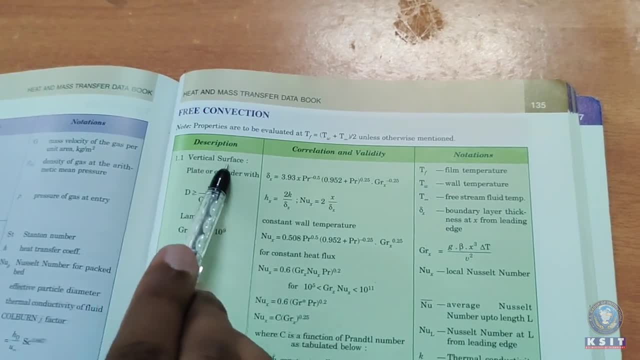 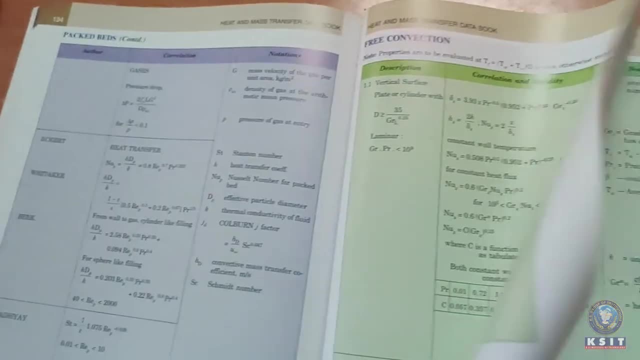 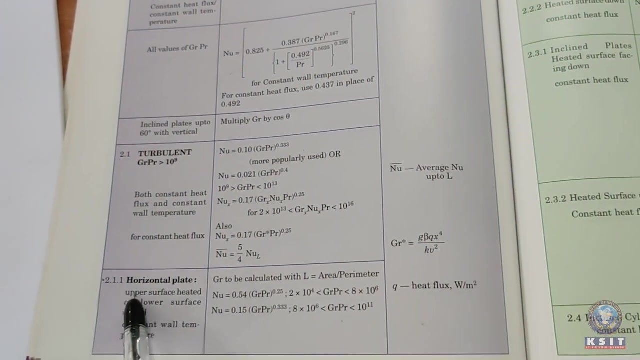 convection right. this one, 1.1, is to the vertical surface. but what we are doing is now the horizontal cylinder cylinder. search for horizontal cylinder right. it's not available in the page number 135, turning page number 136. it's nowhere horizontal plate we got it's not still horizontal cylinder right now. 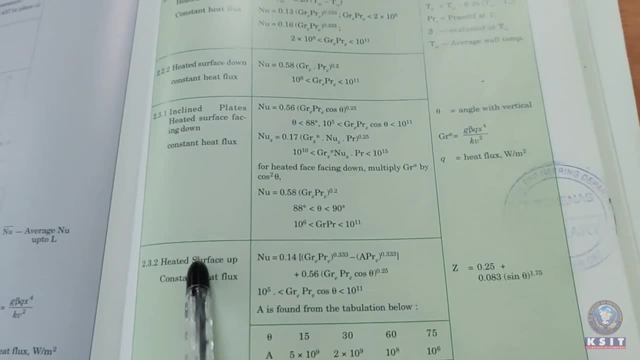 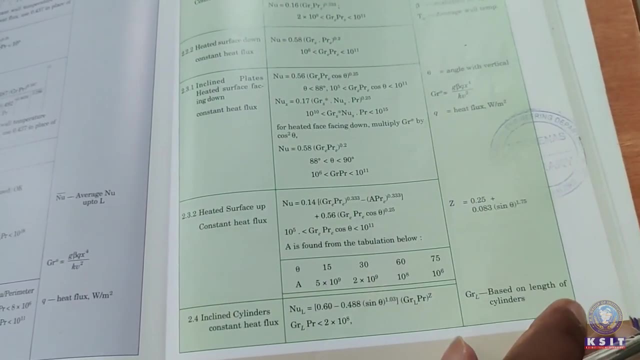 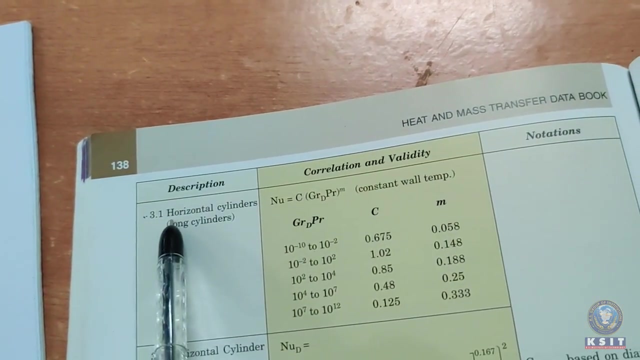 in the page number 137. keep on searching it right. there's a horizontal surface. now we got inclined cylinder right, but what we require is horizontal cylinder right. page number 138, equation 3.1. we should be very happy now we got horizontal cylinder word right, so use this correlation for horizontal. 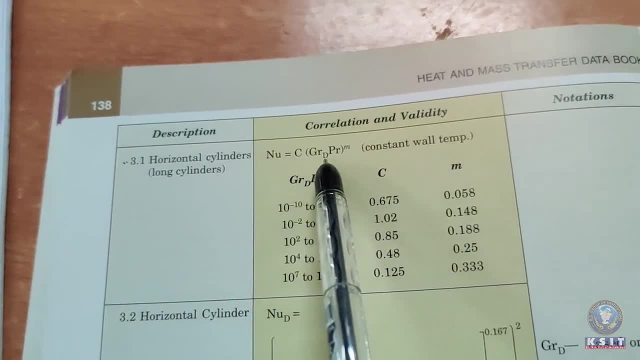 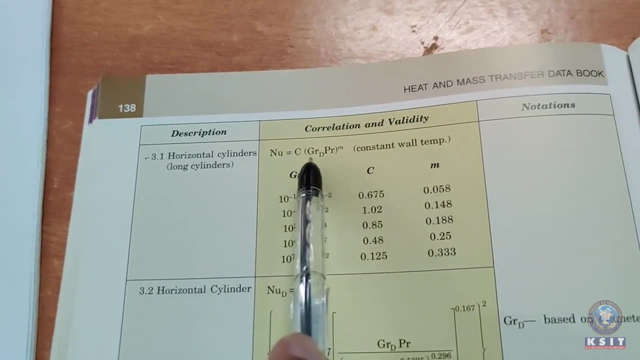 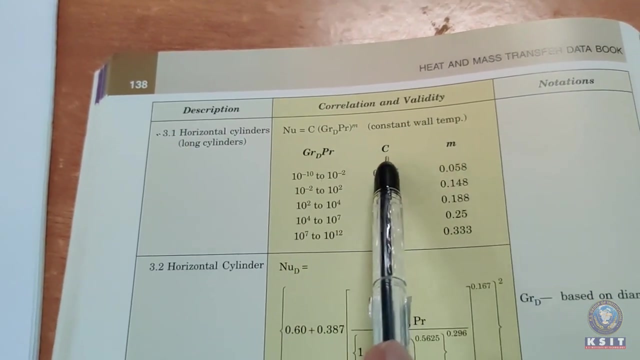 cylinder that is nu, is c, gr, d pr to the power of m, right. so find out the product of gr pr, what we got from the calculations. if the gr pr is in this, any of the range, take the corresponding c and m value, capital c and small m value, right, so find out the range. 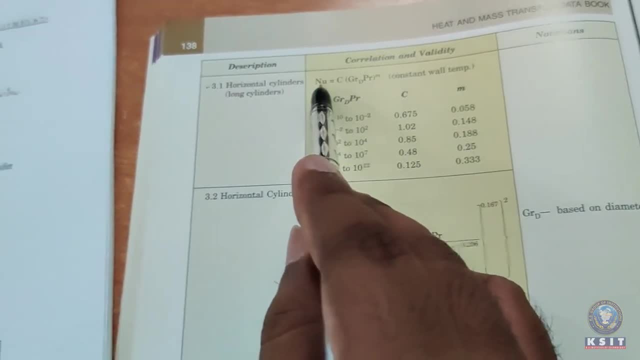 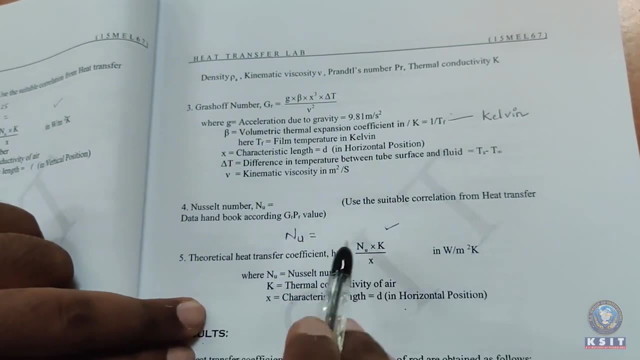 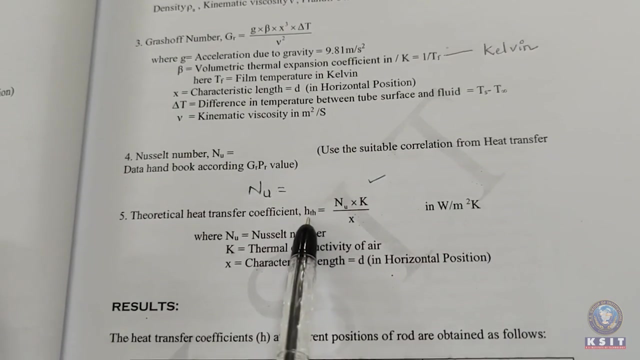 and take these two values and calculate nuzzel's number. nuzzel's number we can get and write, which doesn't have any unit. it is a dimensionless number, right? so, coming back to the manual, find to find out the theoretical value of h, h theoretical, is nu, k by x, nu nuzzel's number, what? whatever we 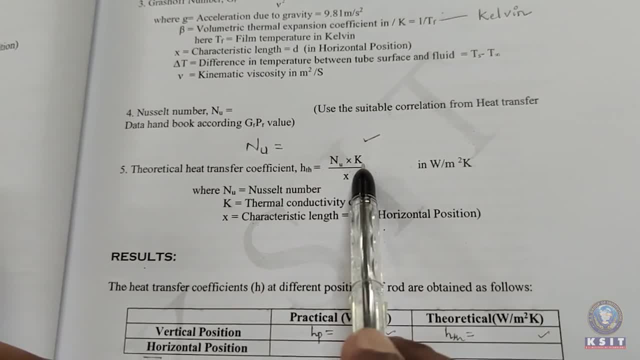 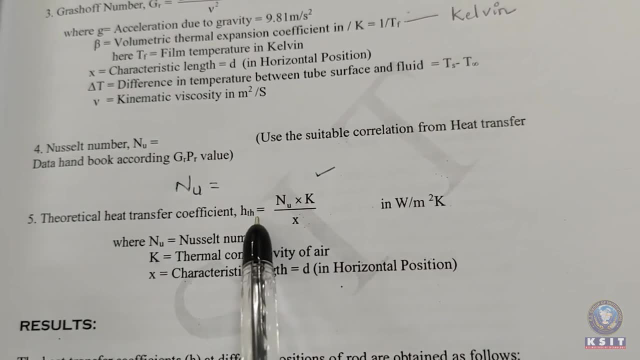 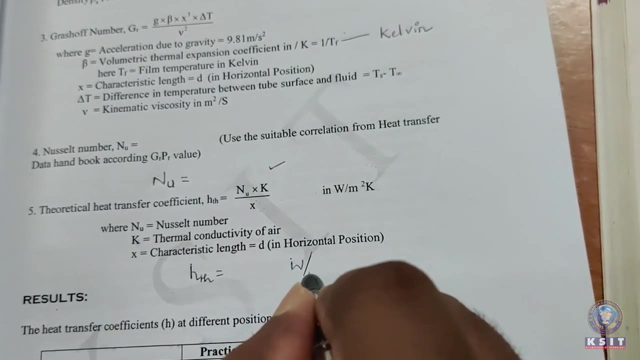 got k value is thermal conductivity of air from the property table. then x is a characteristic land and that should be definitely the diameter of the rod, right. so we definitely we can find out h theoretical, which is for the horizontal position, that is in watt per meter square kelvin, right. so